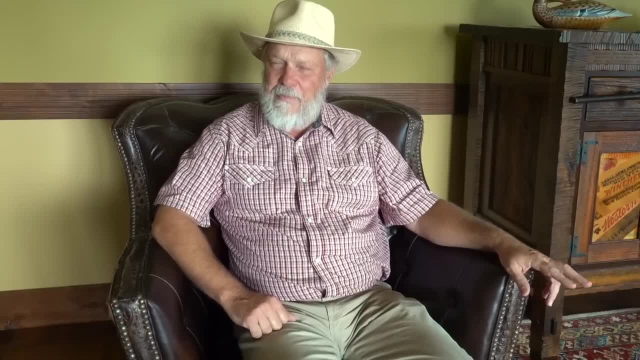 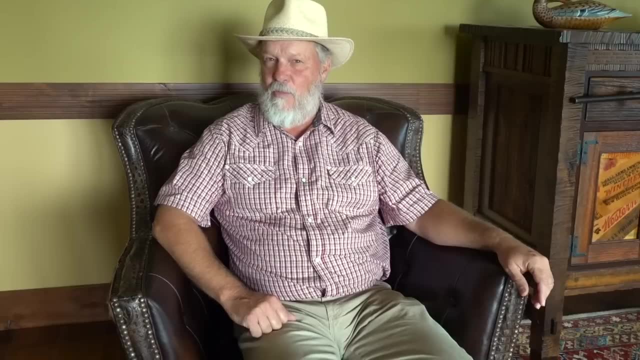 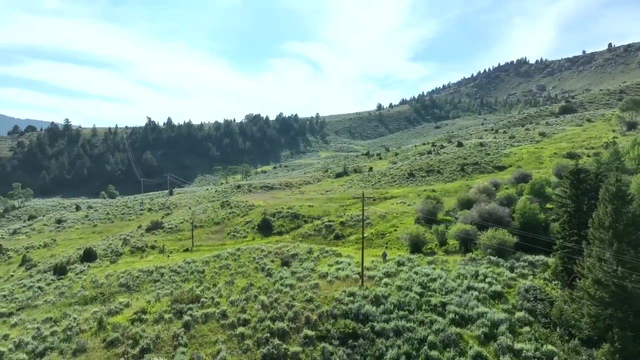 Let's start this process by evaluating two hypothetical properties that you're considering building a home on, Or perhaps they're properties that already have a home on them that you're thinking about purchasing. Looking from above, we see a very nice place to locate a home. 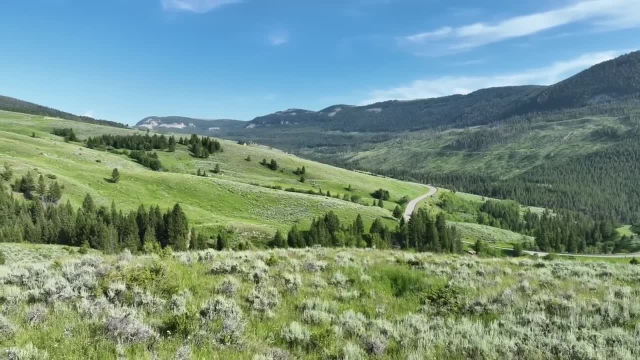 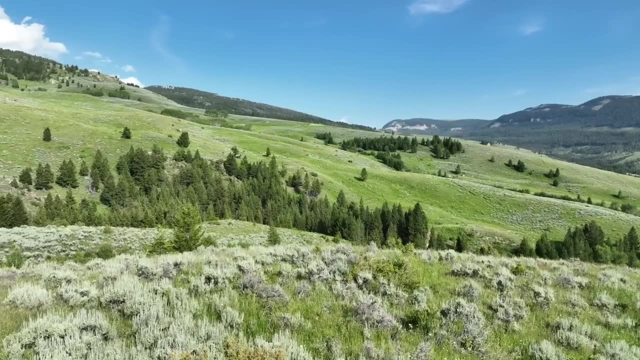 The views down the mountain from the potential home site are incredible, aren't they? The landscape out in this region catches my eye and leads me to think that more evaluation of the area is warranted. There are wonderful views- Views up the mountain as well. 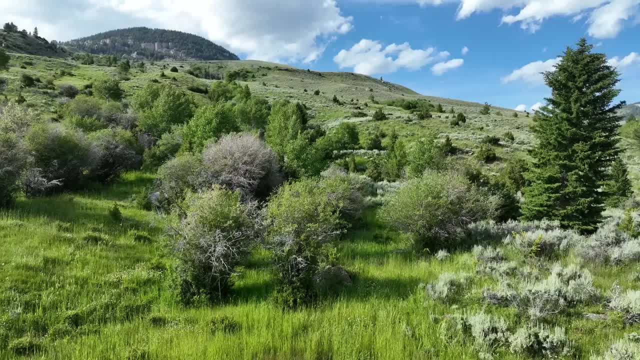 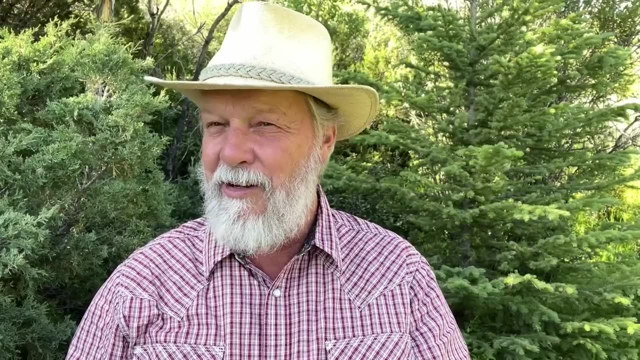 But again, some of the landscape focuses my attention. In particular, up in this region are some features that need to be looked at. One of the things we can do is just send up the drone right here and go from here, from your home site, and look it over from the drone and get that perspective. 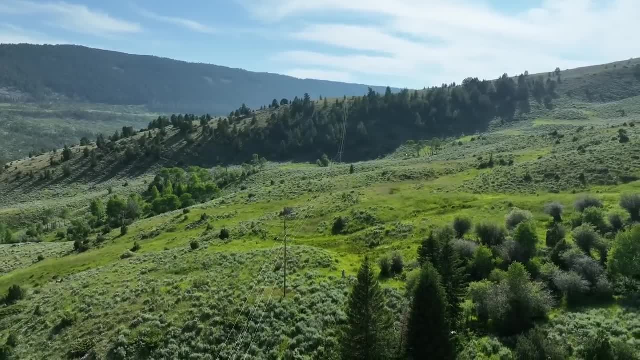 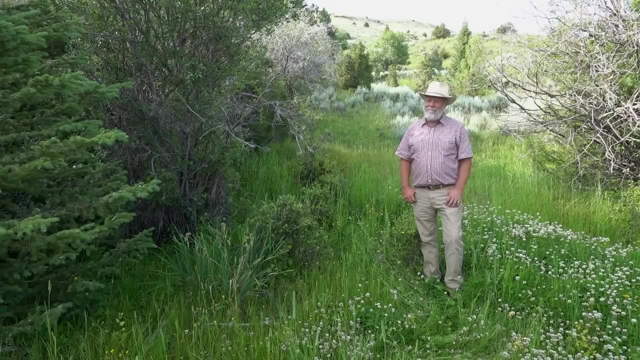 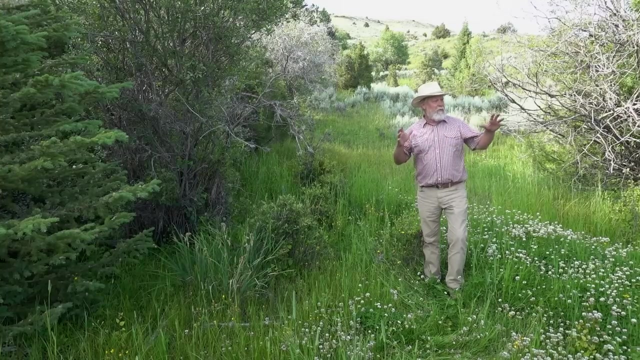 That could definitely be helpful. I did send up the drone. and what do I think? Well, I have some good news and some bad news. The good news first. We can find a wonderful place to build your home on your property with the wonderful, beautiful views of the mountains. 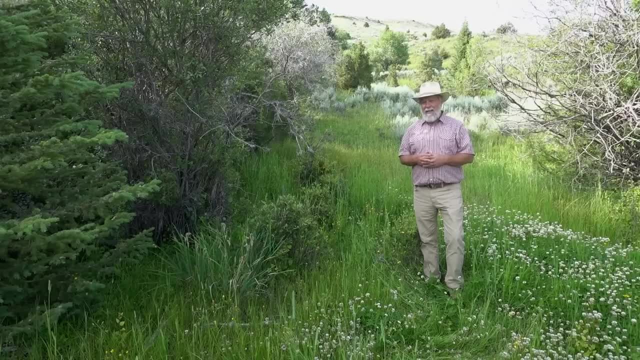 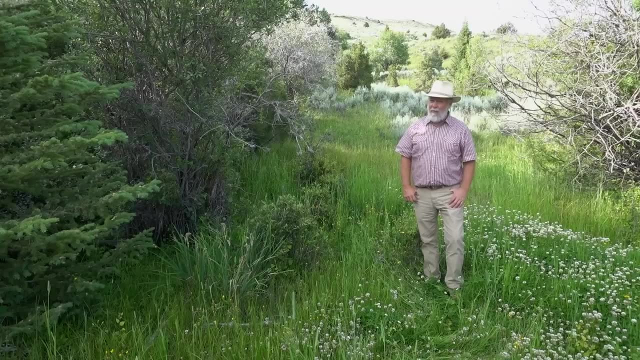 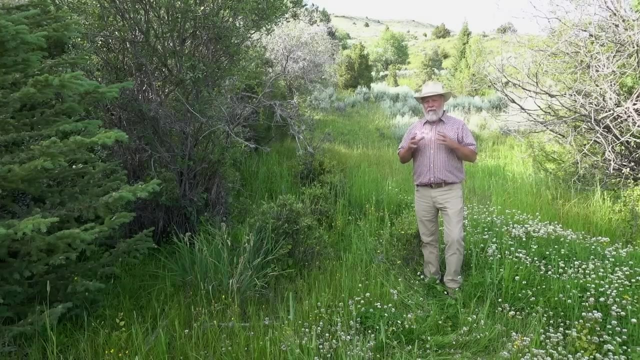 These amazing mountains around you and you can enjoy it here. The bad news is, we cannot build the home where you wanted to, And in fact, there's quite a large area within your property that we do not want to build your home on. I believe that it would create grave danger for life and property. 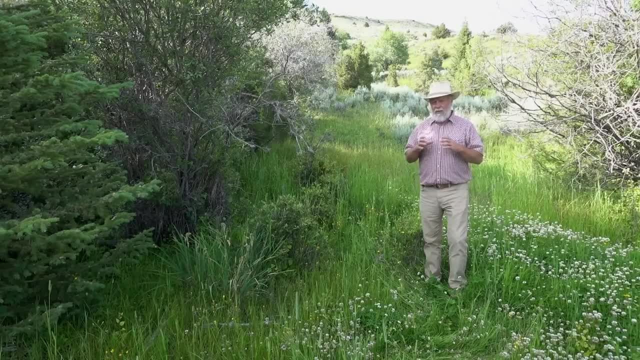 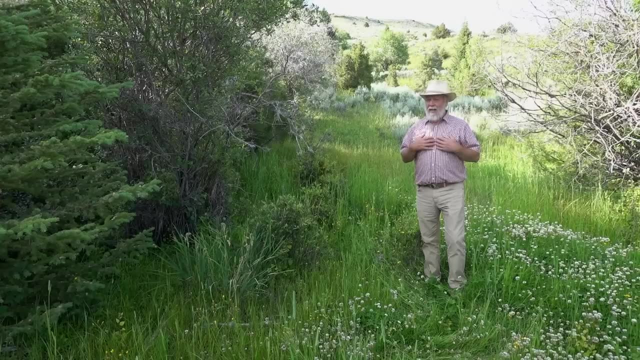 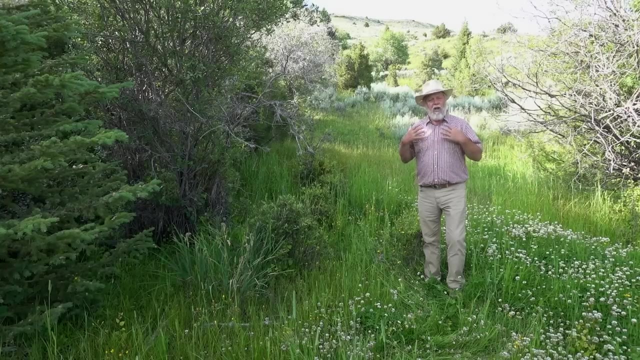 Now. I say that because, as I was recording the drone video and seeing it, I saw several features that were very clear to me that said stay away. So we're going to come back to this drone video later. I don't want to show it to you now without some knowledge first. 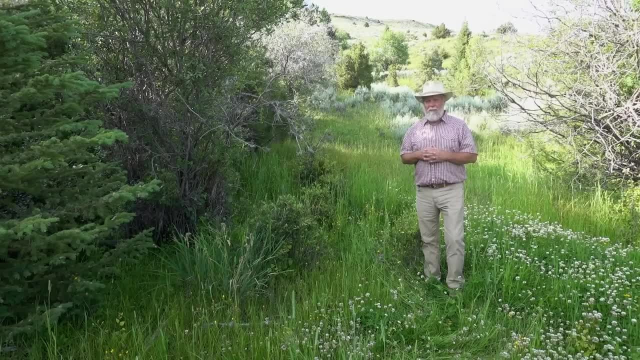 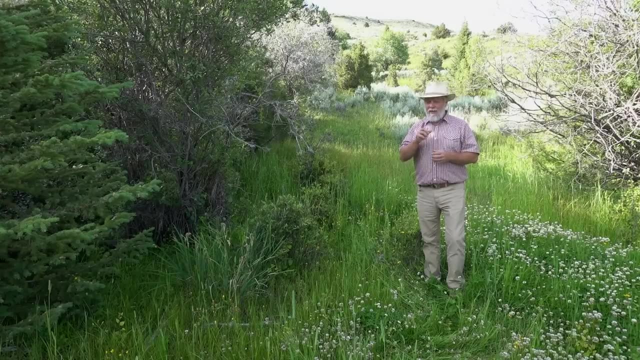 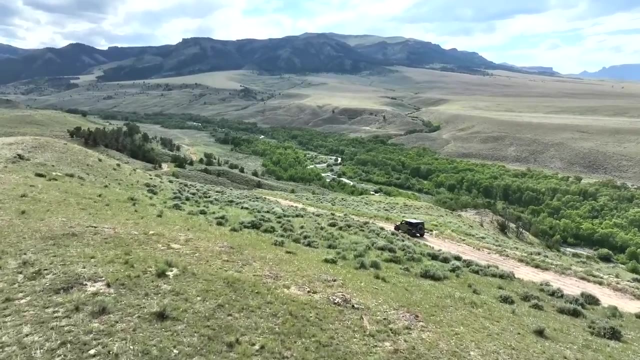 So let's go forward and learn more about landslides and mass wasting and all that, And then we'll come back and see this drone video And I think you're going to see immediately the concerns that I had. What I love about field geology is it gets you outdoors exploring areas that are often overlooked by others and help you visualize our wonderful Earth's history. 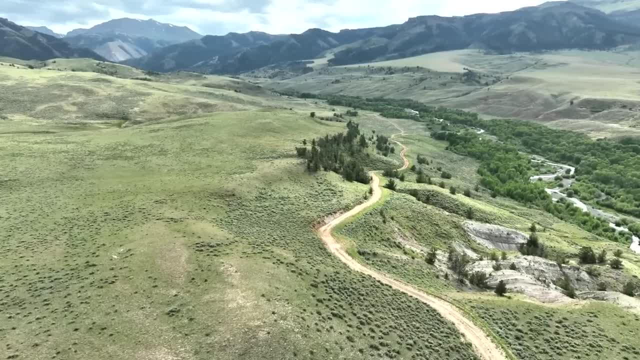 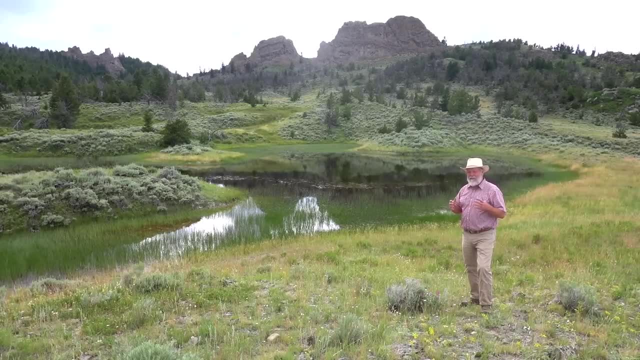 The adventure I'm having exploring landslides is no exception. I'm excited to see what lies ahead. Well, I'm having so much fun thinking about potential home sites, I thought I'd show you another one. This is really a nice area. 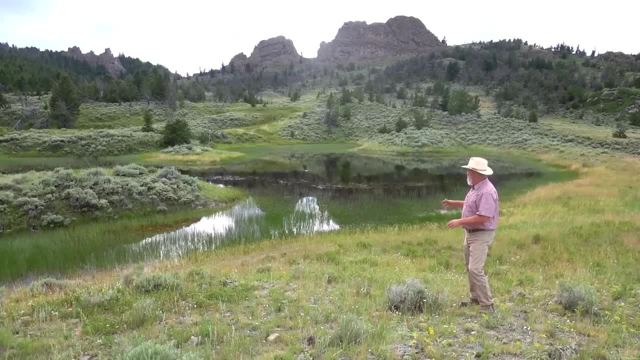 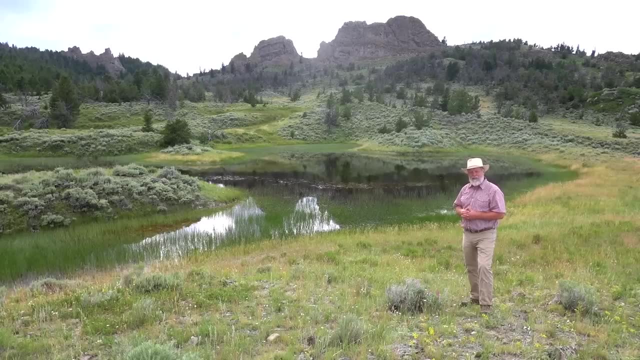 We've got a pond here, with a little hill in the pond, interestingly, And there's several ponds scattered about which you'll be seeing, And I want you to think about this as a potential home site, right about where the camera is, right where you're looking at me right now. 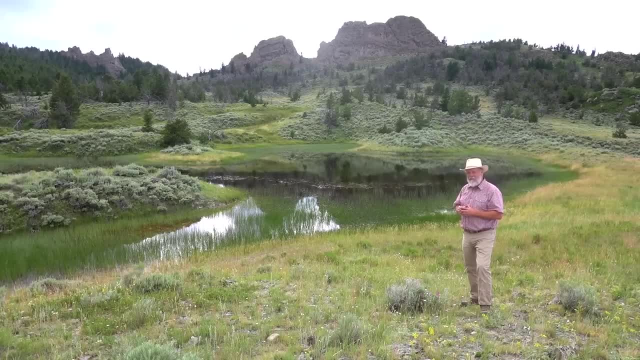 And you'll have the opportunity to evaluate this more carefully. I'm going to show you a 360 view so you get a feel for the area, kind of low down, as if you were standing here, And then later I'm going to show you a drone view where we back out and see the big picture and let you evaluate it after you have more information about what to look for in landslides. 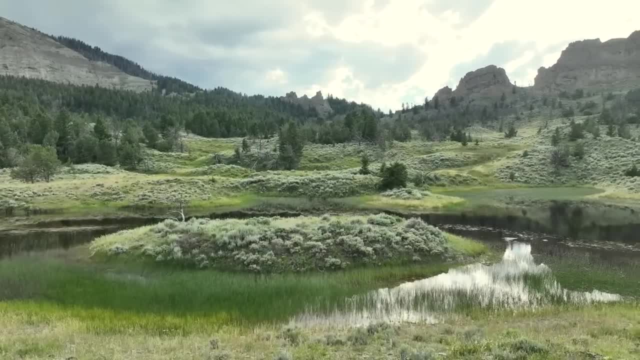 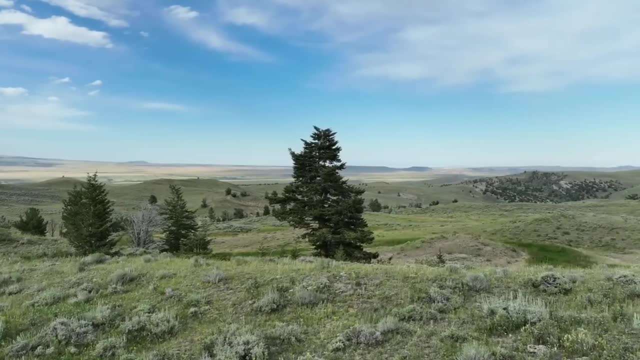 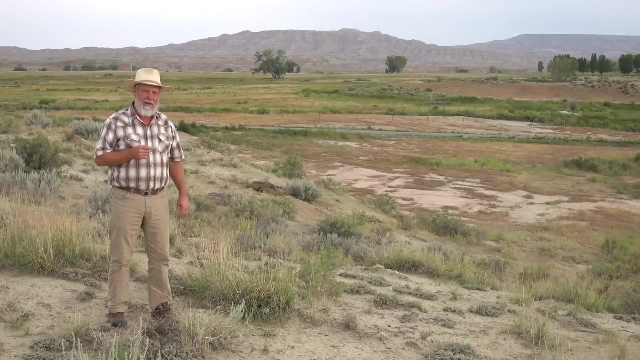 Looking up the mountain, you couldn't ask for nicer views, could you? And turning around and looking down the valley, the views are just as spectacular. All of us can easily recognize modern landslides that have occurred, But the key to staying out of trouble is the ability to recognize ancient landslides that have been heavily eroded and weathered. 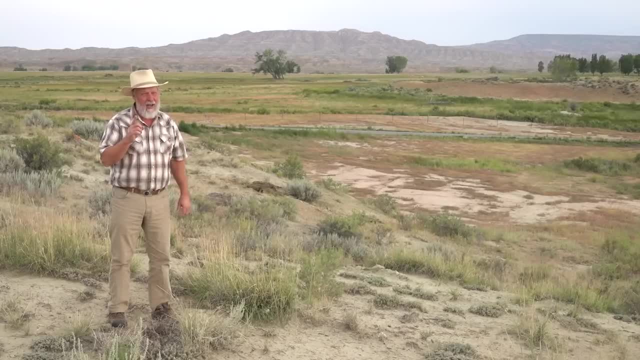 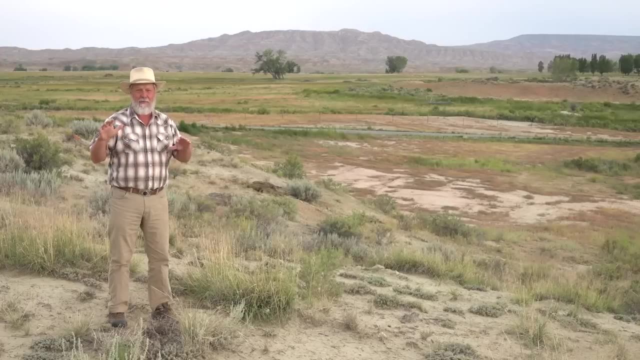 Now, why would I say that? Well, it turns out, with very few exceptions, wherever there's a modern slide that has occurred, you can be sure that there are many ancient landslide scars and hints of those landslides in the same area. 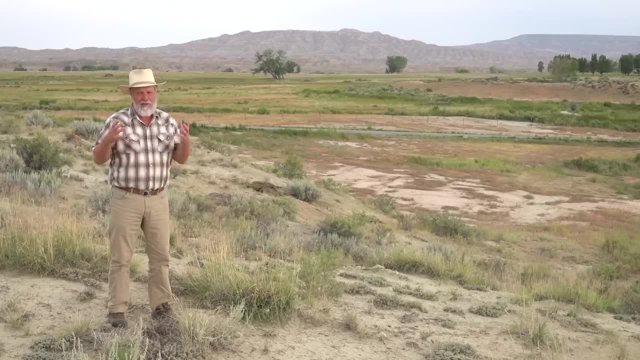 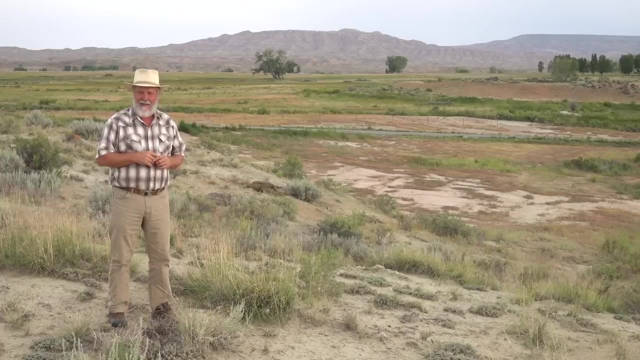 So this is a fairly simple concept. If we can just recognize the old, we know that we're at some risk of something occurring today. But of course, in order to have this ability, we need to have a sound understanding of landslides in general, especially the modern ones, and then learn how to recognize these. 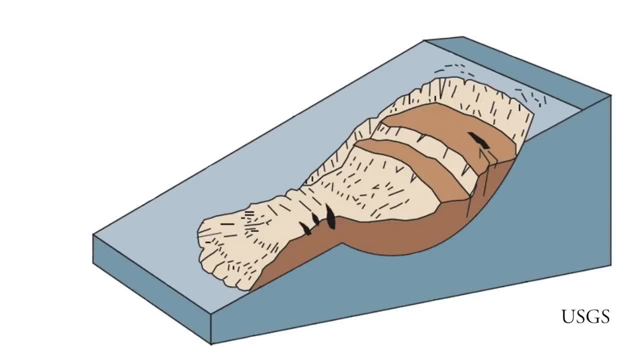 There are several different types of landslides, But we can use this illustration to understand some basic features. Here is the surface of rupture, which is a fault and is often spoon-shaped. At the top of the slide, the break forms a steep cliff face that is referred to as the main scarp. 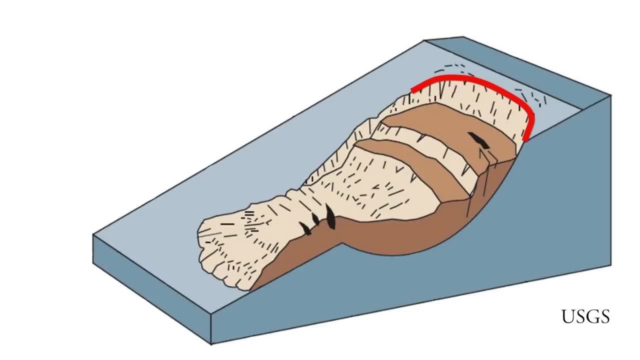 The top rim of the main scarp is very commonly arcuate or bite-shaped. It's not uncommon to have multiple scarps. We see a second one in this illustration. I like to refer to these relatively flat areas shown here and here as benches. 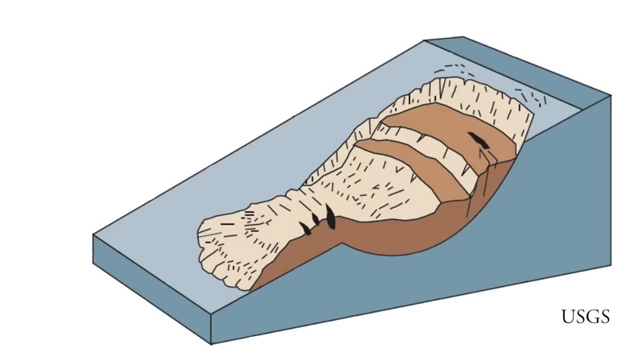 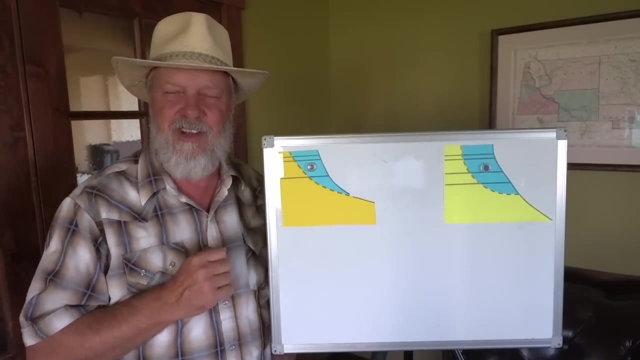 They often dip back towards the hillside. At the bottom of the slide is the toe, which often behaves more like a debris flow, And the small black lines represent fractures. Okay, so over to my handy whiteboard to help us understand these landslides better. 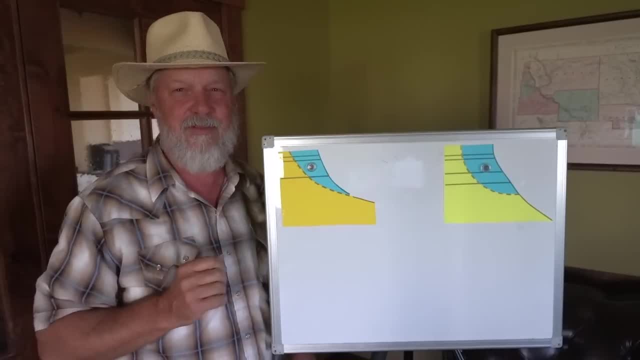 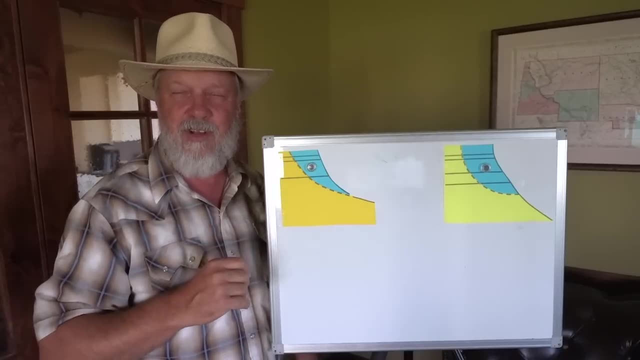 I have two models that I want to show you. There are many different types of landslides, but I only want to focus on a couple- end-members, shall we say. I may mention some of the other types later, But let's focus on these. 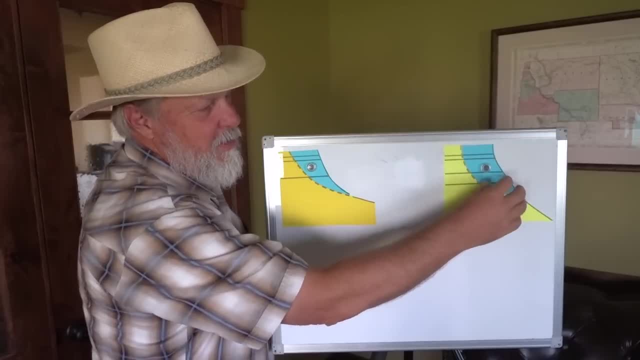 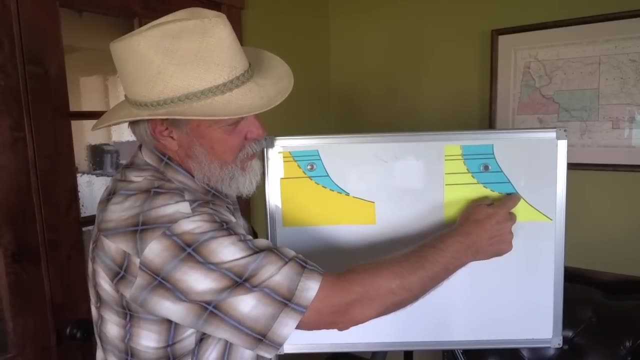 First of all, I want to go to this one on this side. The blue part of this paper or this paper model I have here is the piece that's going to break free along this fault here or that rupture zone we've mentioned. 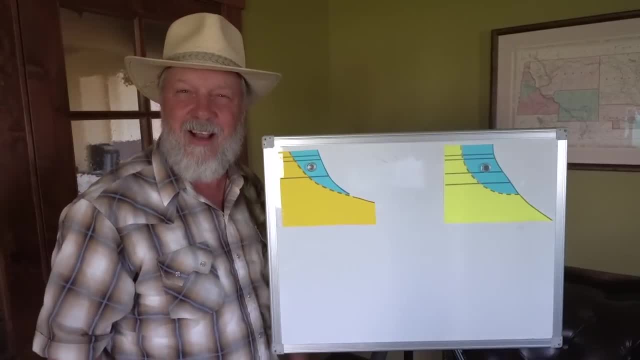 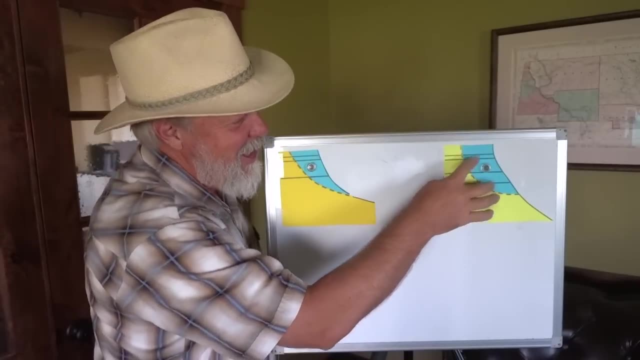 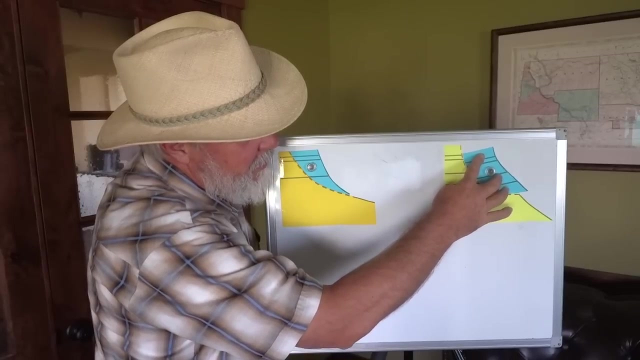 The horizontal lines represent the layers within the rock. So as this breaks- and hopefully your home isn't sitting right up here, for sure- as this breaks and it rotates because of the shape of this, it just kind of immediately starts rotating as it slides out. 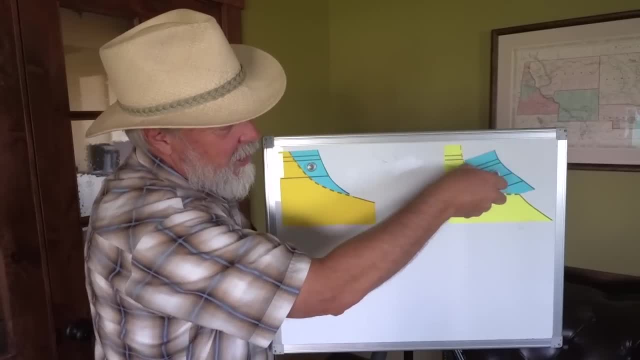 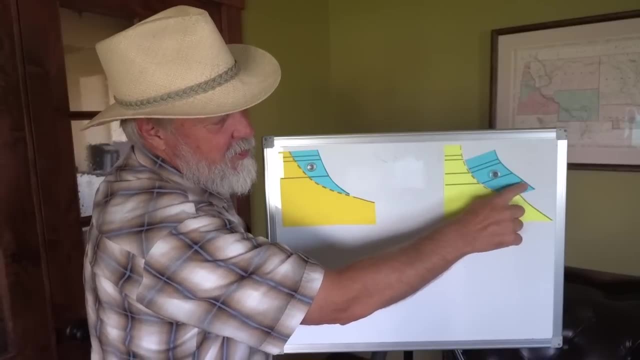 And see what's happening. As it slides, these layers are rotating and dipping back into this fault surface. Now out here, of course, this is going to start breaking up, And what not as well. It doesn't hang out over like this, of course. 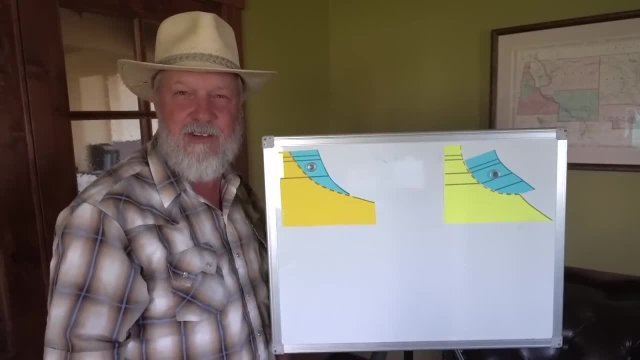 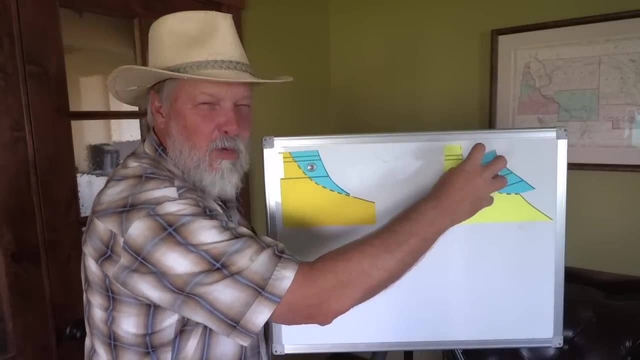 It'll fault and flow and all kinds of things happen out there as well that I'm not going to get into. The main point is it's rotational and you maintain more of a block-like status. Okay, now to discuss this side here, this other end-member that I want to discuss. 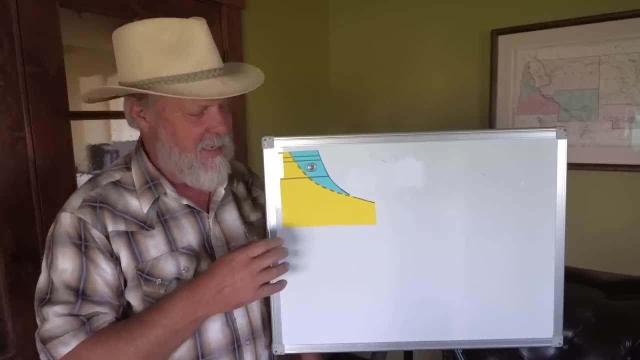 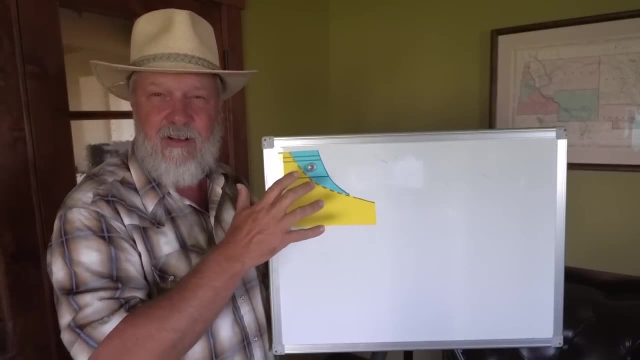 I like to refer to this as the slumping model. We'll call it that. Now, the shape of the fault or this rupture surface is a little different here, And the behavior of the rock, of this block that slides, changes because of that. 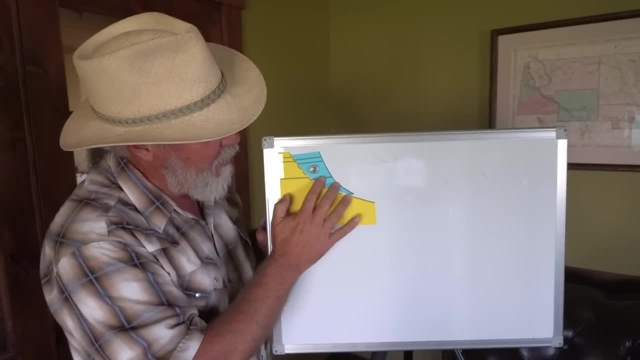 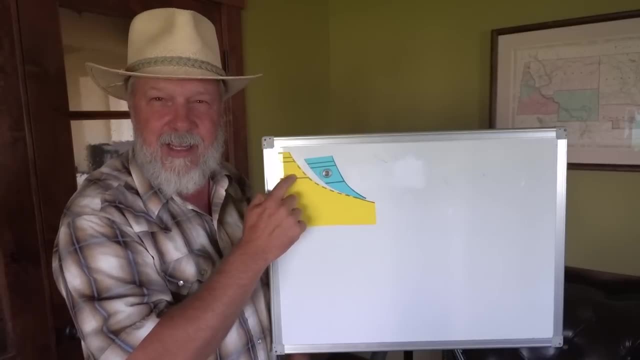 Watch what happens when I slide this out along this fault. here like this, There's, in theory, a big gap that's forming between this block that's sliding and the Mother Earth. I'll call it over here And of course that can occur. 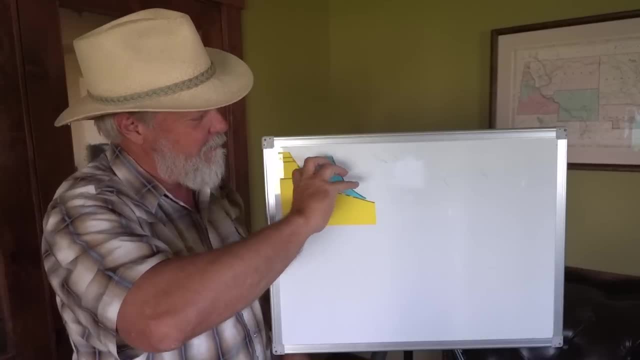 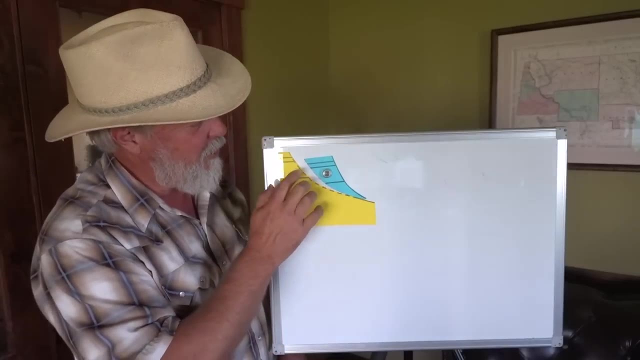 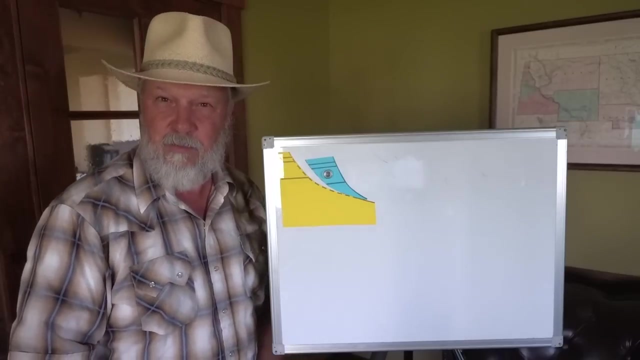 It bends and deforms and folds back in. I don't want to fill that hole there that I've got here. You never have that gap. So what does it look like? Well, you have some rotation and some bending, And let me show you a quick sketch of what it does look like. 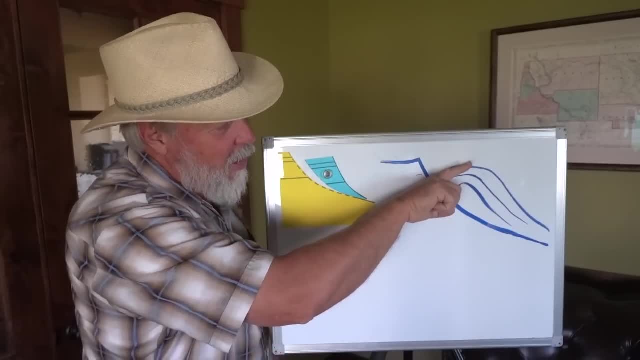 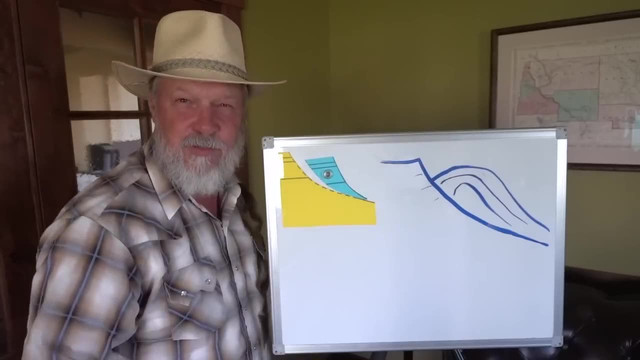 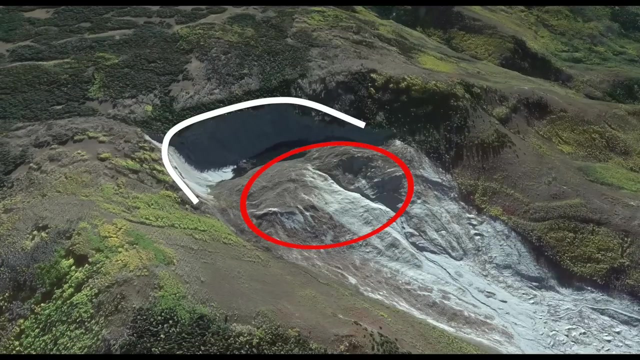 And so we have this folding. But notice all the rock, the layers and the mass of the surface dips back towards this fault. Here is a nice example of a large slump Showing the headscarp and the rounded hill below it. The gray color is caused by thousands of dead trees. 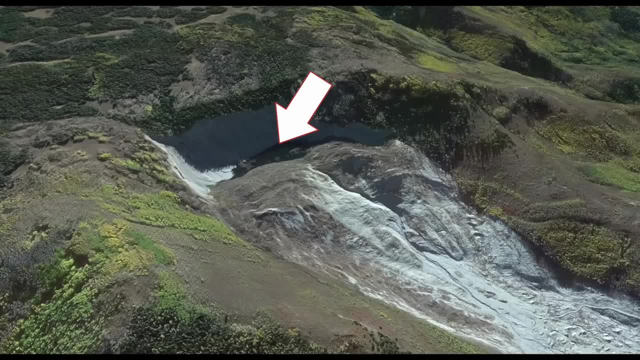 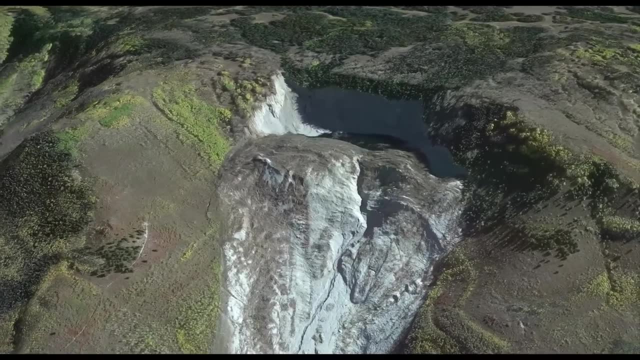 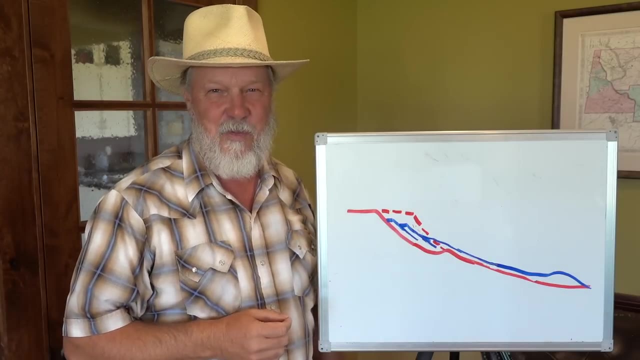 If you look closely, you can see a small lake or pond back in the shadows. here In large landslide complexes, there are often many of these hills of various shapes and sizes scattered about. Okay, another sketch on the whiteboard to help us out. 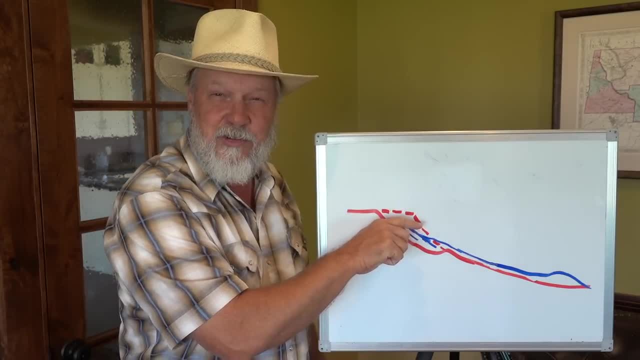 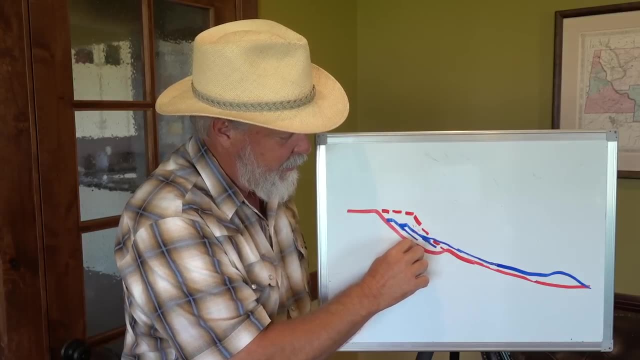 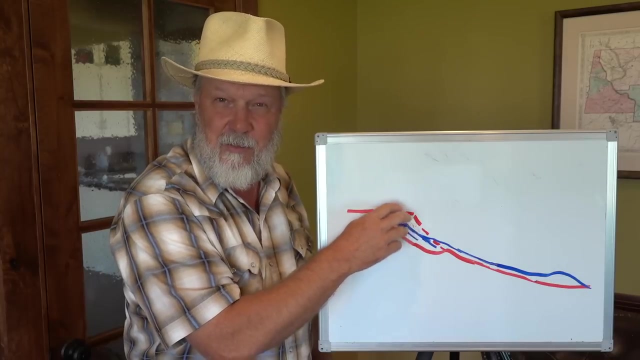 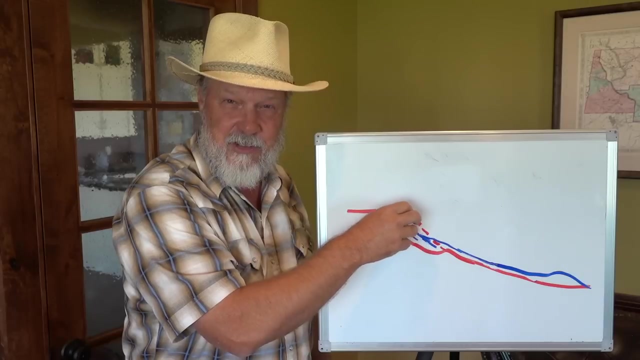 This dashed red line shows the land surface prior to the landslide occurring. The blue is the material. The blue down to this red here is the material within the landslide that occurred. So I've depicted some slumping or rotational blocks here. Now it's fairly common for, at the base of these slides, these slumps or rotational blocks to develop into a debris flow. 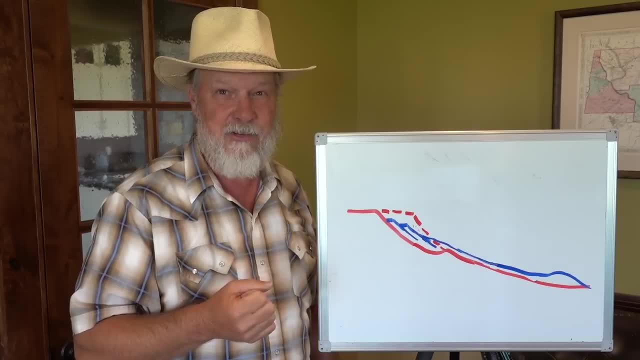 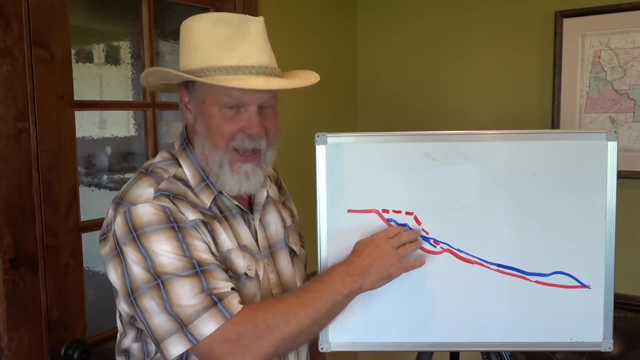 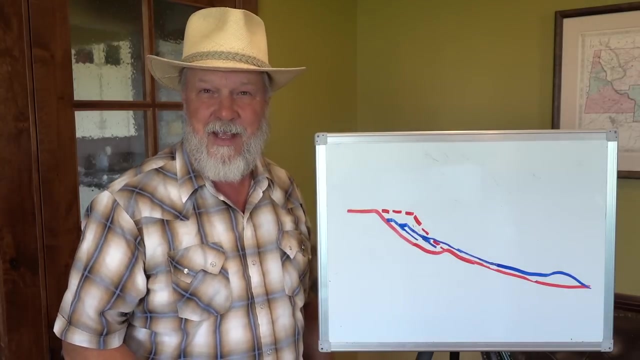 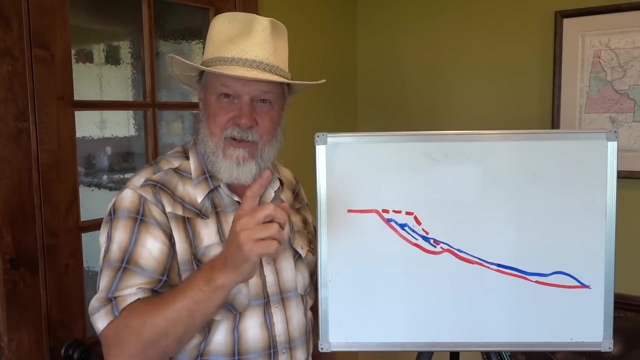 Which is kind of scary because they can move up to 35 miles an hour and run out down the mountain several miles. So here the land surface has dropped, Here we've deposited material on top of the original land surface. I was hiking in this area, right here where the land surface has dropped some, and moved out and found something interesting. 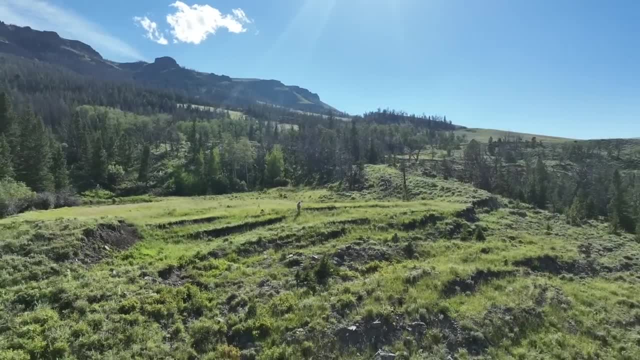 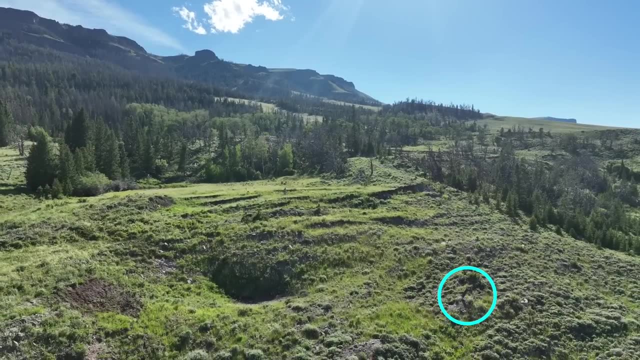 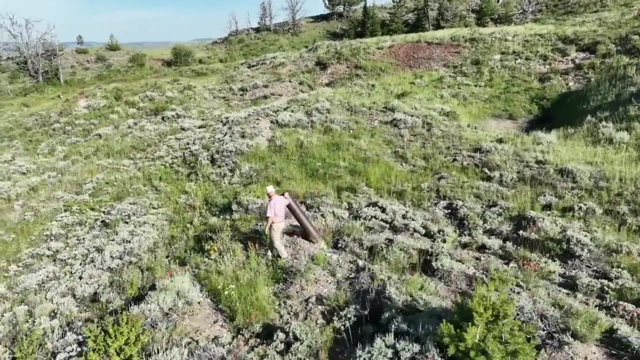 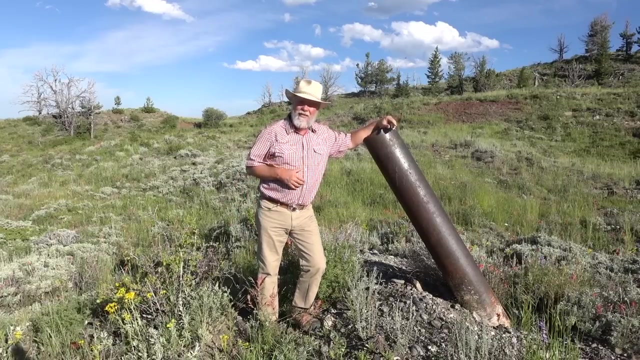 Let's take a look Here we see that the earth is being torn apart. It's right here, but it's hard to see. Let's look closer. Sometimes you get really lucky and you have something that helps you understand the processes involved. 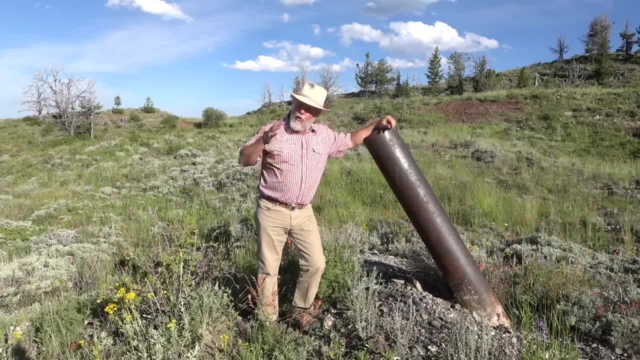 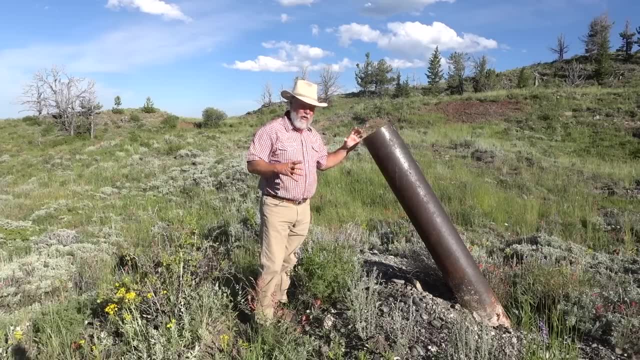 the forces involved and how quickly they can occur. This is a steel casing of a. well, It looks like it's half inch steel, really heavy, and look how much it's bent over. So we know the slide is moving that way. 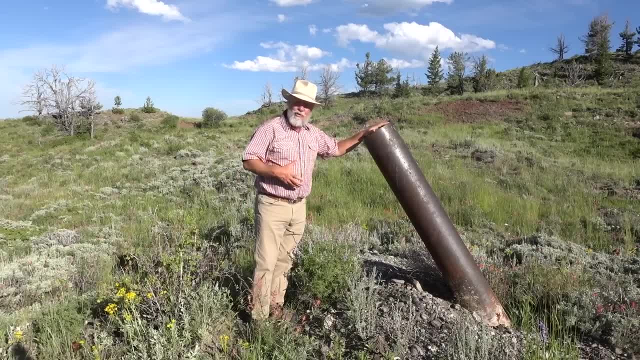 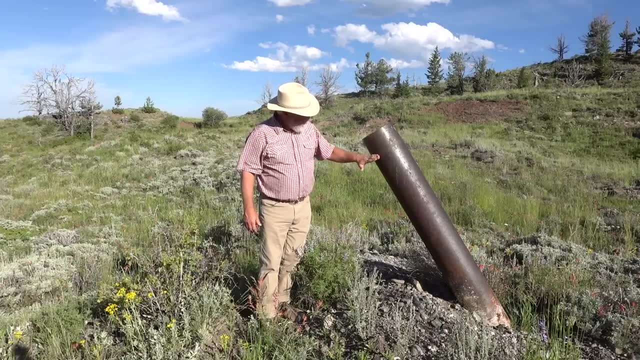 That's fairly obvious, but the forces involved in here to bend this over. And then another fascinating thing is: at the time that this well was abandoned, the dirt was. the ground level was probably about to right here, So the whole surface has dropped down. 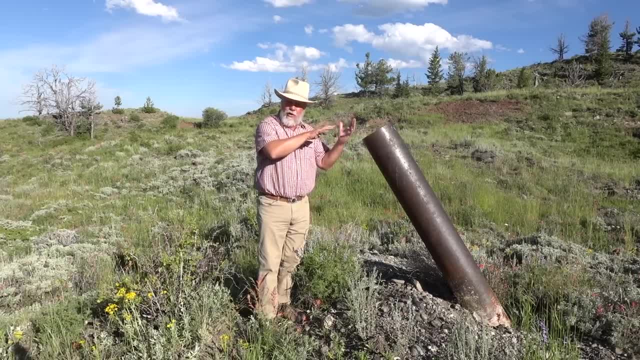 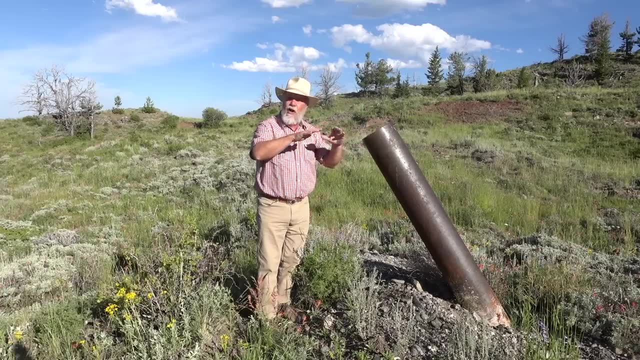 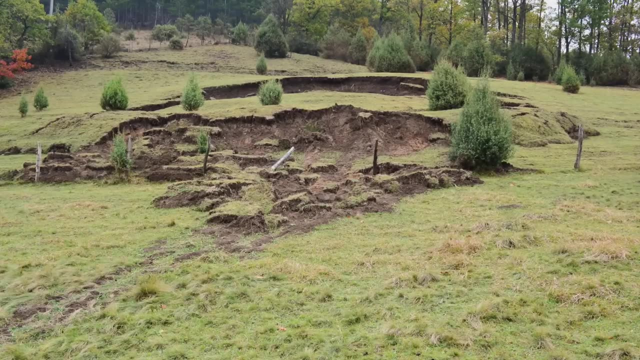 And that's what happens during slumping events and creeping events and slow landslides- well, fast ones too- But the whole surface of the ground, on average, is dropping and moving out. Let's examine some examples of modern landslides. This is a small scale slump. 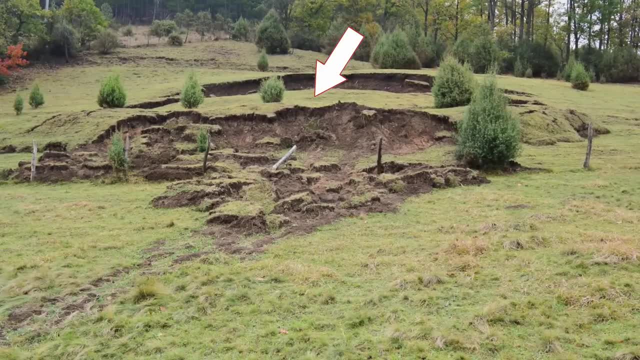 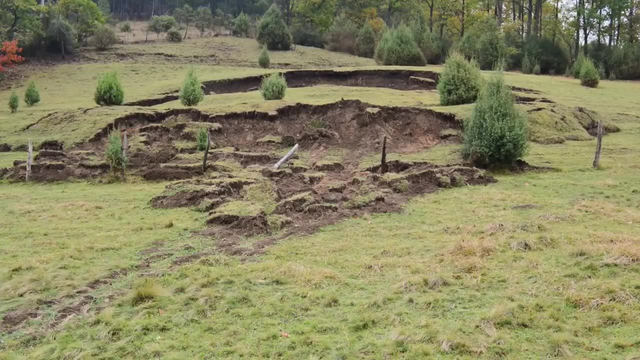 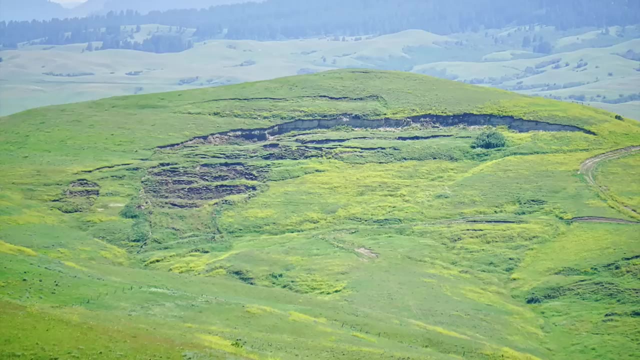 Two bite-shaped scarps are easily seen, with a bench between them. This one doesn't show any evidence of fluidization and therefore develops slowly, likely over a few days. Notice that in this case the slope of the land is quite low. Here we see a small one on a relatively modest slope. 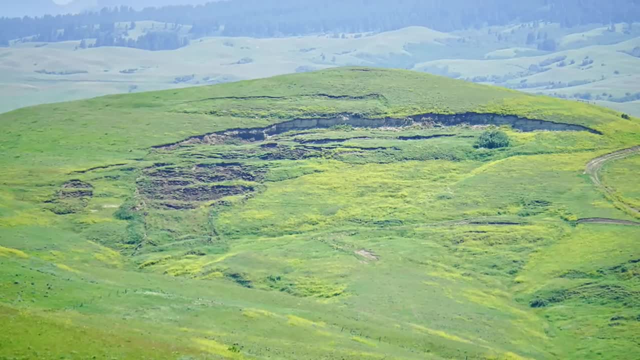 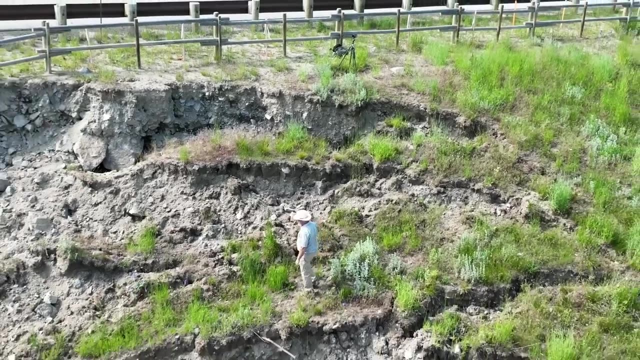 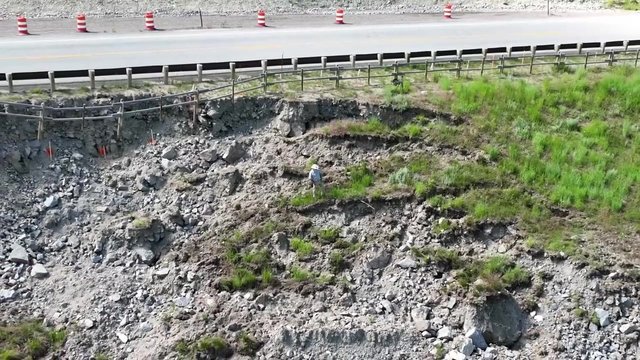 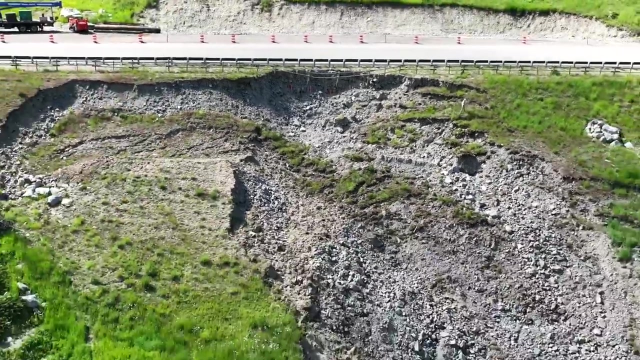 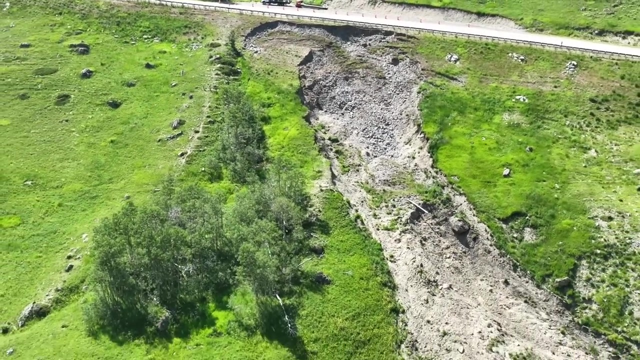 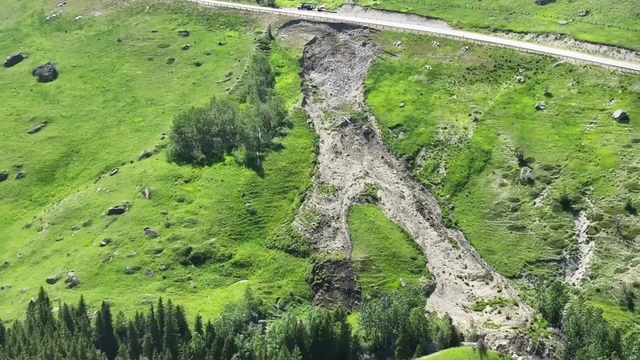 The headscarp is easily identified, along with several benches on down the slope. There are indications of minor flow in the lower area. This one is an example of a landslide that immediately fluidized into a debris flow. Although relatively small, it could easily destroy homes and even threaten life. 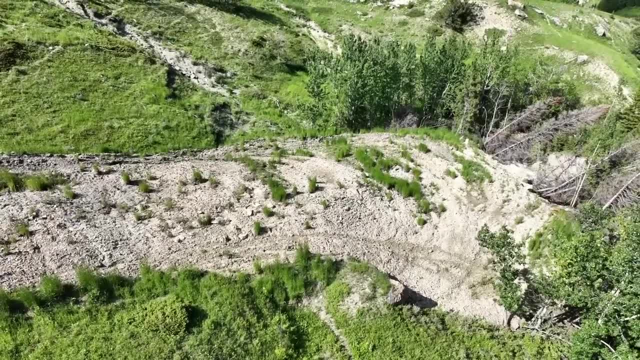 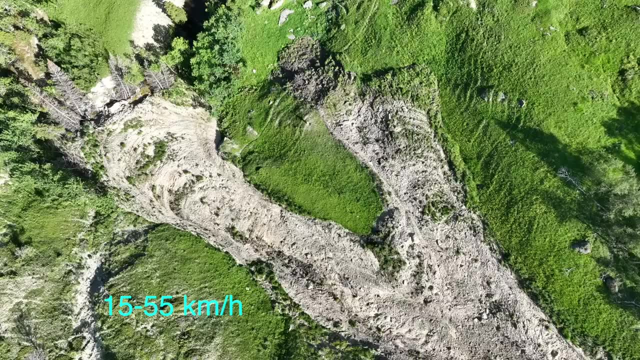 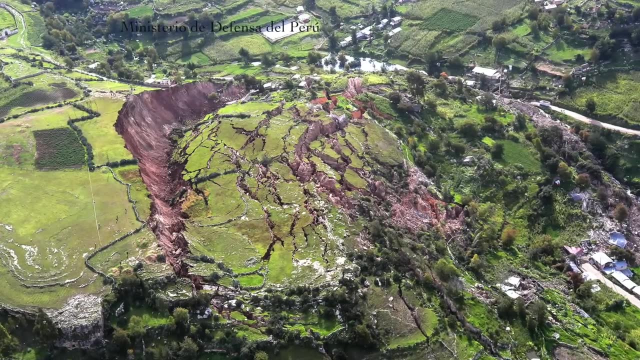 Down at the toe of the slide, you can easily see a series of small arcuate ridges indicating flow. This likely came down the mountain at tens of miles per hour. Scary. This huge landslide in Peru is a classic slump feature in that you see how the surface that we see in the green grass here. 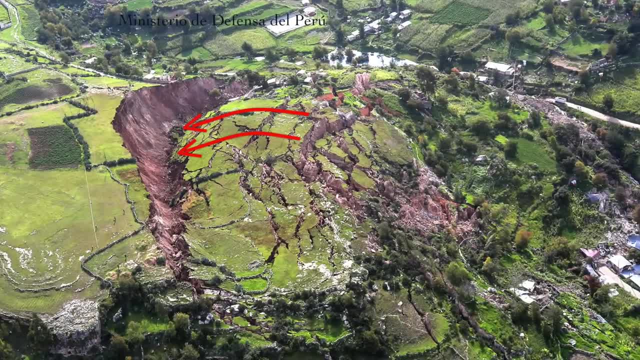 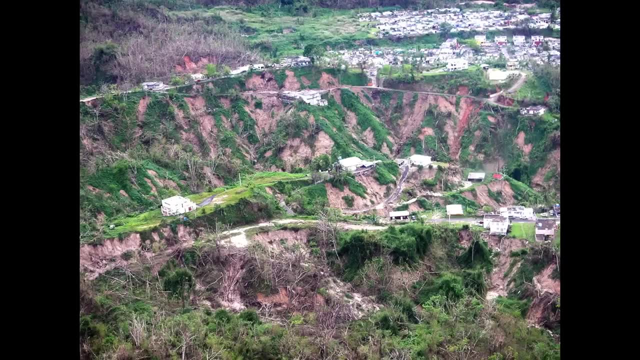 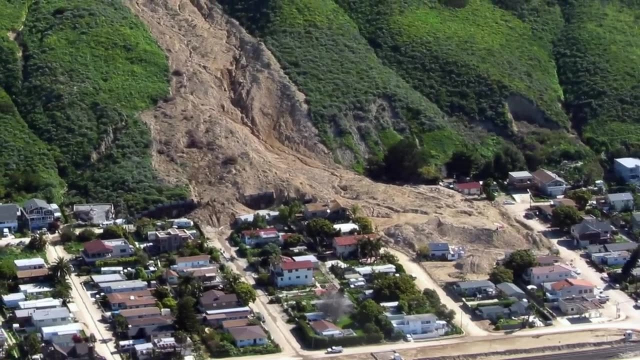 has rolled back into the main scarp And this large landslide in Puerto Rico shows several large blocks with benches on top that work down the slope. This one occurred in La Conchita, California, in 2005.. It was likely a slump-like feature that immediately fluidized into a dangerous debris flow. 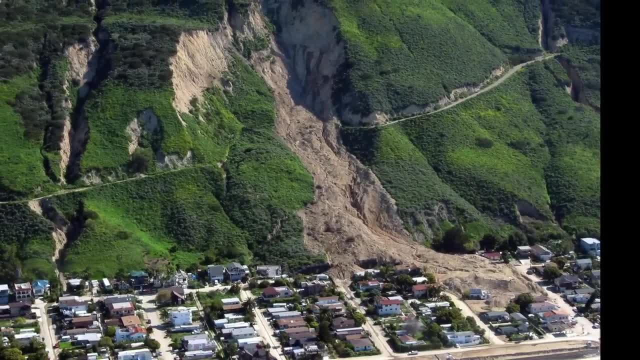 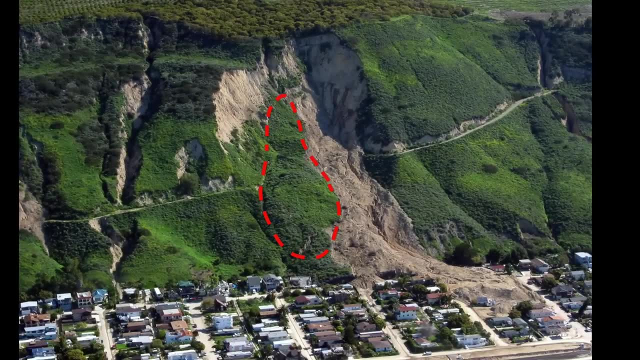 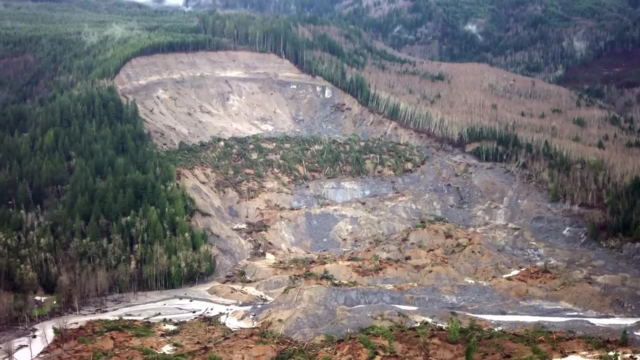 It killed ten people and destroyed many homes. Interestingly, there was a prior slide in 1995, seen on this slump-looking feature covered in grass. This is the infamous 2014 landslide in Oso, Washington, that killed 43 people. The area was known as Slide Hill. 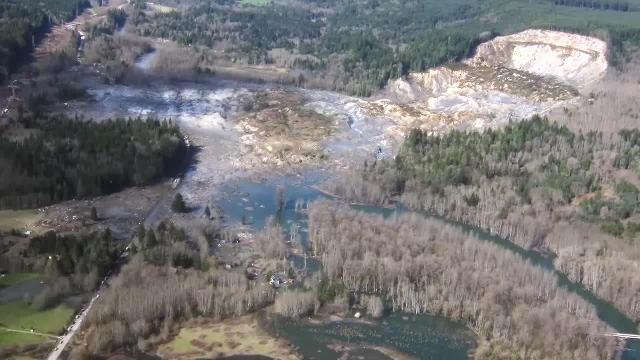 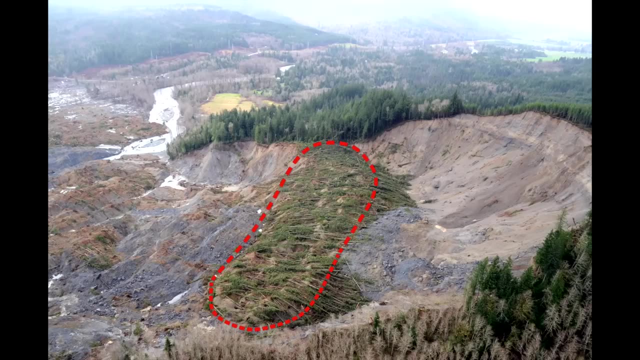 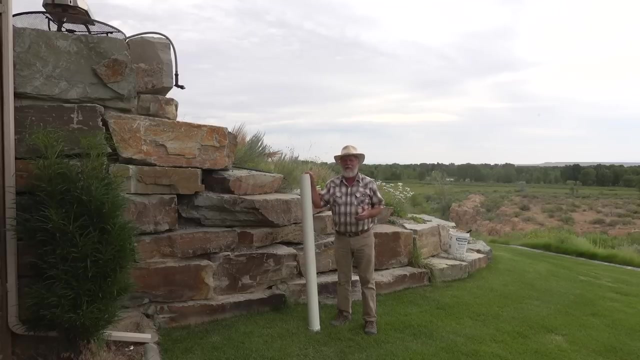 and there was at least one significant slide in 1962. on the same slope. You can see one large bench and other small ones on down the slope. Unfortunately, the lower part fluidized into a deadly debris flow. So now that we've seen examples of modern landslides, 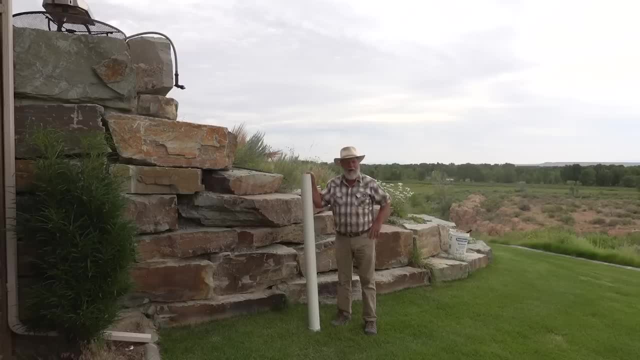 and we understand their features pretty well. the obvious question is: why do they happen in the first place? What is it that triggers them? And that's why I have this pipe here you're probably wondering about. I've got it sealed off at the bottom. 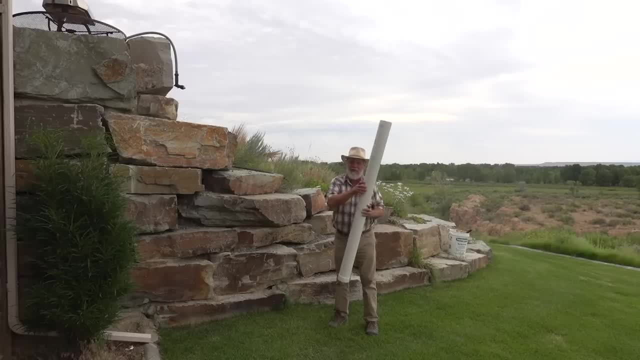 I have a small hole drilled here and this is going to help us understand this better. But first let me talk about the conditions necessary. Number one: slope. Yes, the steeper the slope, the more likely they are to occur. of course, 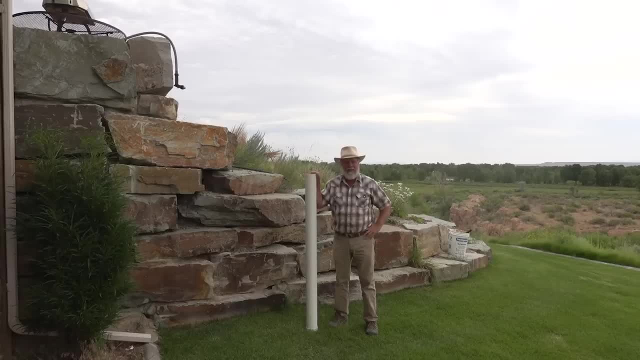 But we've seen that they can occur on fairly modest slopes. The material involved, if it's unconsolidated, it's not as strong. And you add water into that and boy, it gets really weak. A shale can be very prone to this kind of landsliding we've been discussing 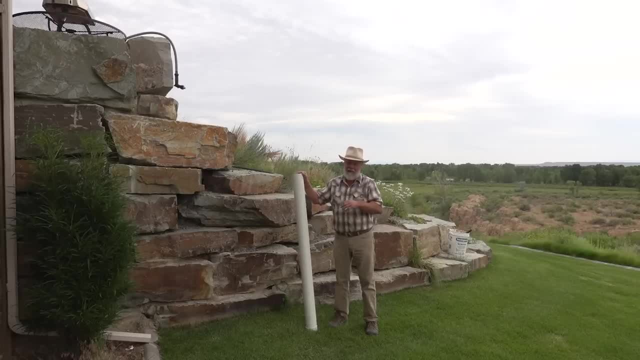 I'm not going to talk about rock avalanches, which are very different, where you have hard rock that just crumbles off a mountainside. We're talking about these that are more fluid or slumpy. Okay, so, with that information, we come to number three: water. 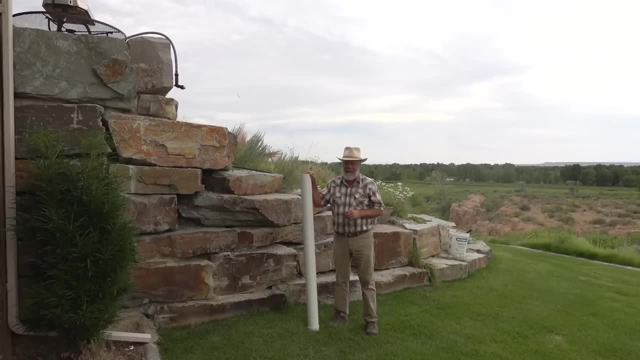 And I've alluded to that. Water is the key And, in particular, if you have poor pressure. And what is poor pressure? That's simply pressure within the spaces between all the grains of rock You have spaces, or pores, You put water. 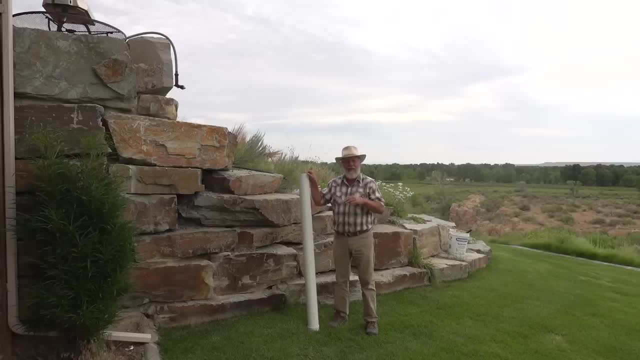 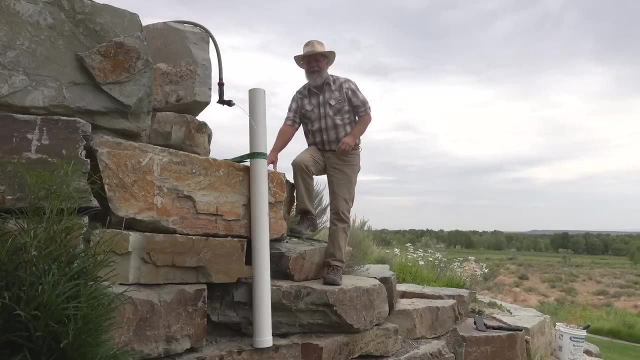 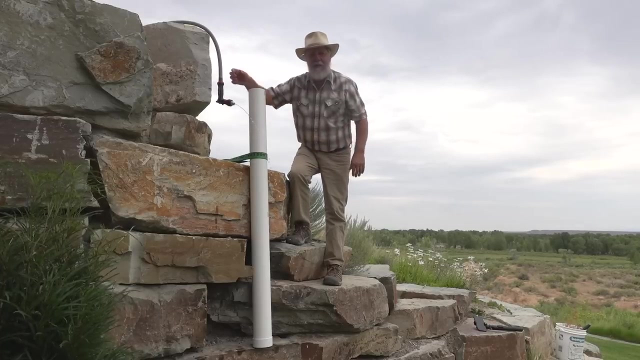 If it's fully saturated, you build up pressure And it's equal to the pressure of the water column or the height of the water table. So I have a hose here with just a trickle of water coming out. I'm going to put it in the pipe and let water run out of the small hole in the bottom. 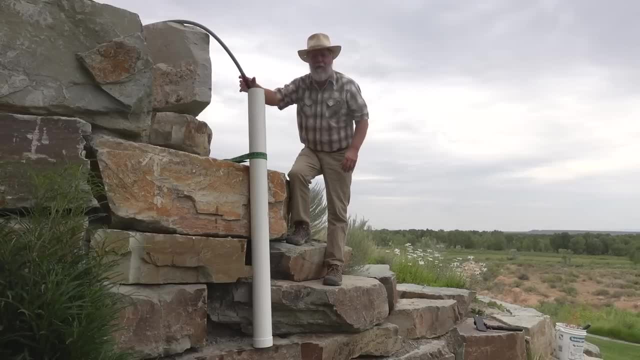 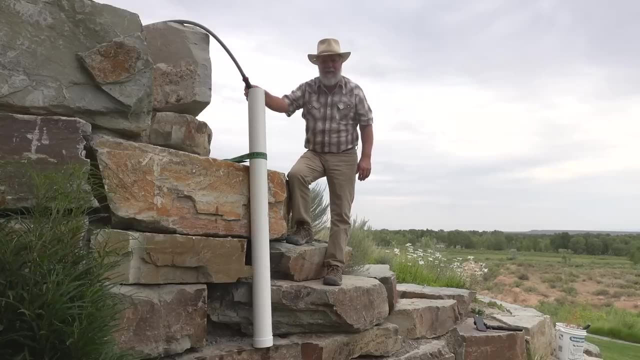 We're going to reach an equilibrium or a balance where the water going in equals the water going out. And since I'm not putting much water in here, I'm never going to develop a head of water here, It's just going to kind of trickle out like we see. 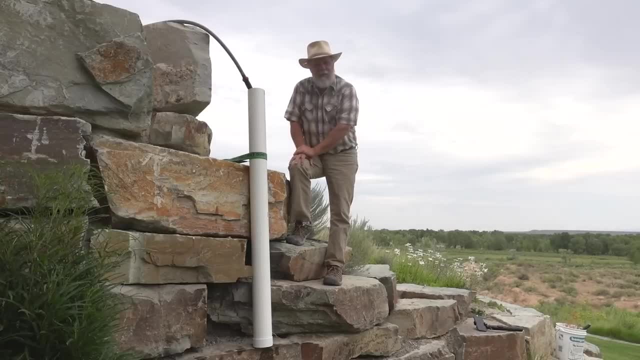 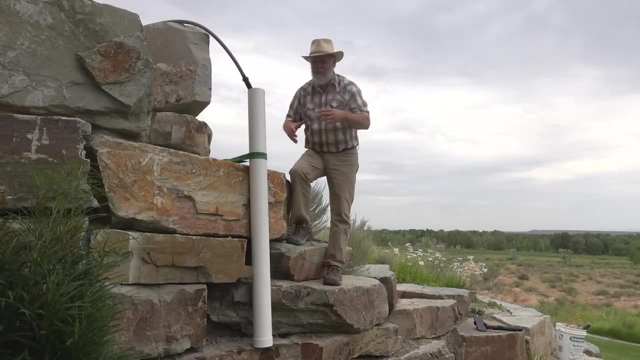 Now it turns out there's a natural balance in landslide prone areas. So if you're looking at a landslide prone area and you see signs of seeps and springs, that's just telling us that there's this balance occurring where the water in equals the water out. 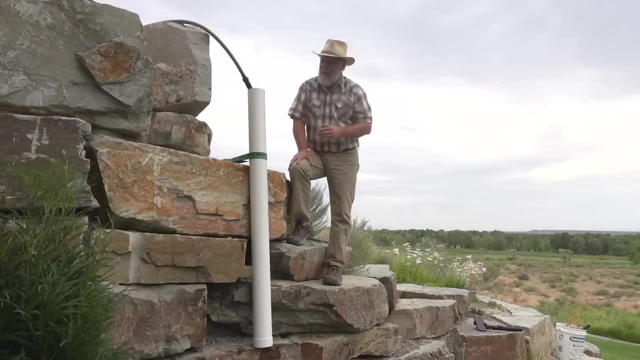 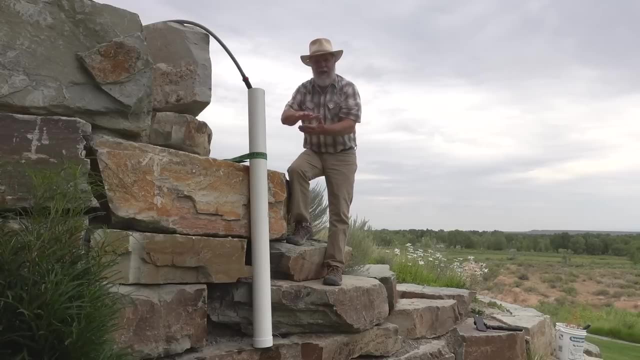 And we're never really developing a column of water. Now, if you get a lot of rain and you start putting a lot of water into the system, then you start building pore pressure that I talked about. It's at 0.43 psi per foot. 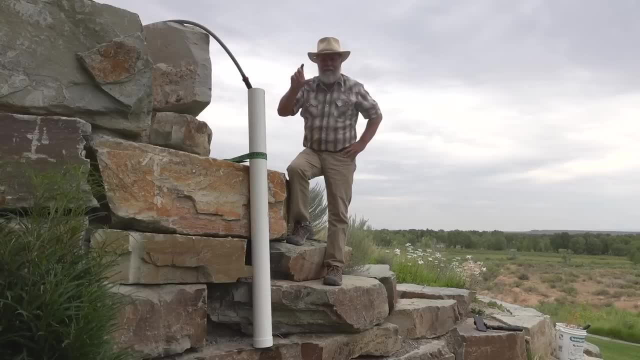 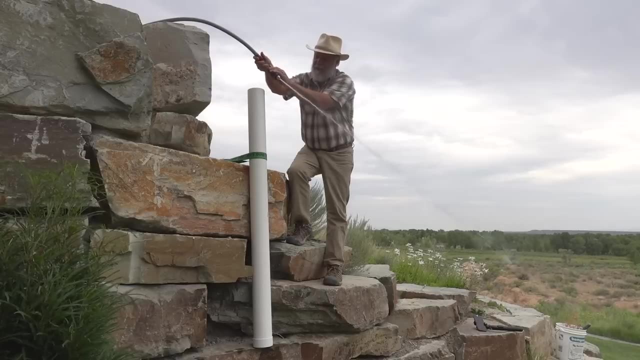 For this guy it's 5 feet. If I let it build up to 5 feet, I have 2.1 psi. Let me do that. So I'm going to turn this all the way up And I'm going to set it in here. 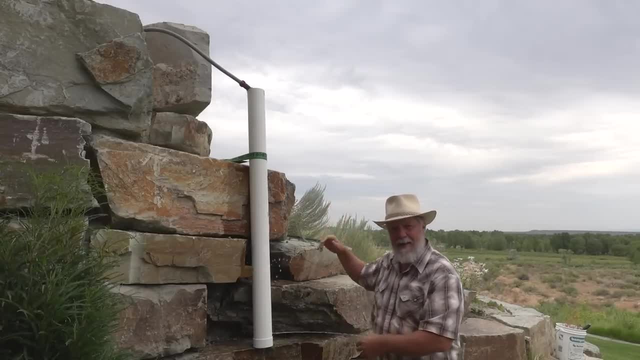 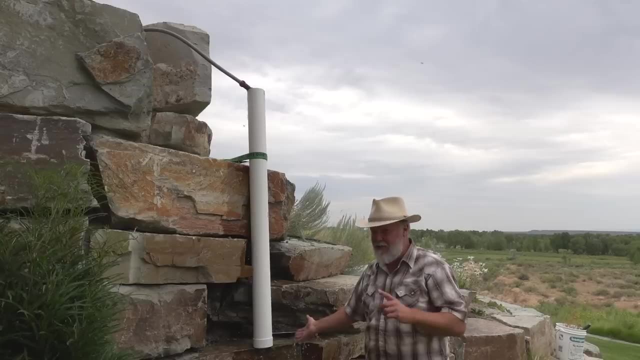 So now we have it running out of the top, We've got the full 5 feet. We have 2.1 psi here, Boy, it's more pressure than you'd think. This is really significant, even at 5 feet. 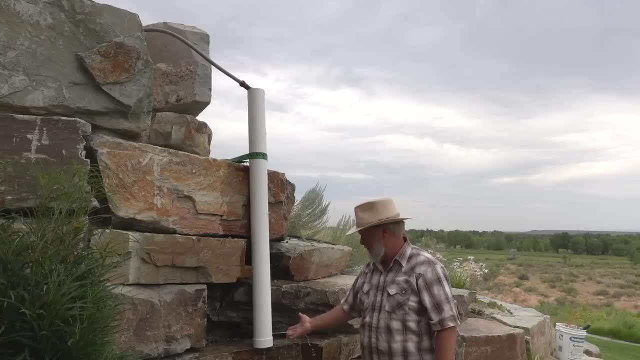 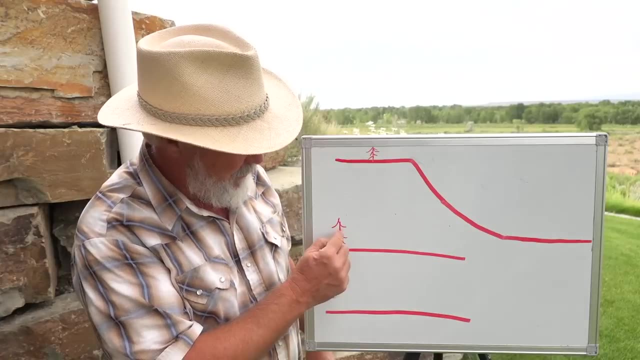 Whew, I'm getting a little wet To my handy whiteboard. to help us out here, I want to focus on this lower part first. I have my famous tree here, to make sure we understand, we're looking sideways. cross-sectional view. 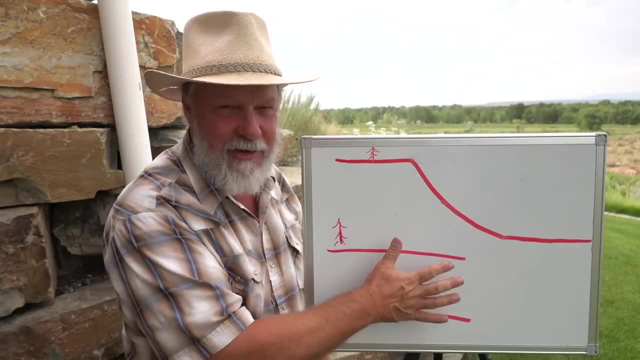 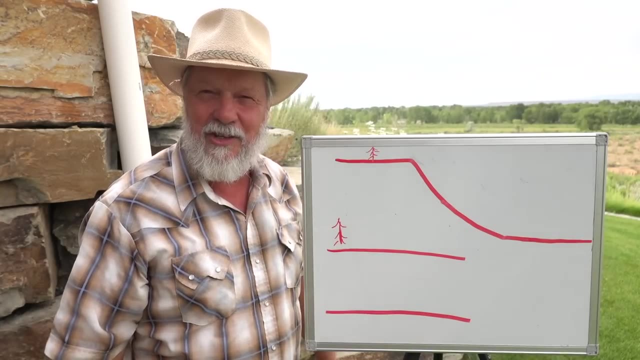 Of course this is the ground surface and I've just drawn a line here to show a line within the ground, And let's assume it goes for a long ways as far as the eye can see. essentially, Now, if you have rock here, which is often the case- that can contain water, you can build up water tables. 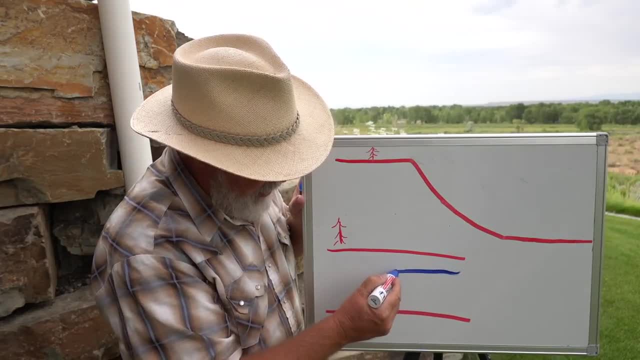 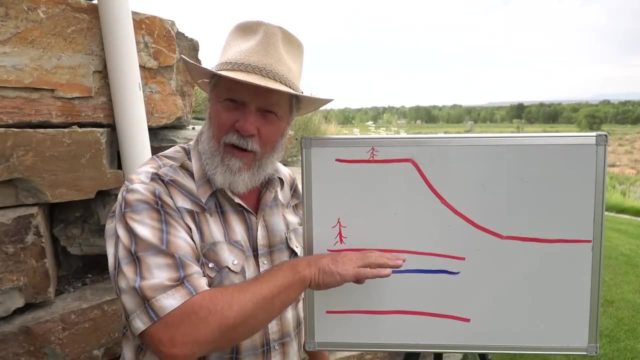 And so I'll draw one in here. Let's say it's right here. So the water table is defined, as I've mentioned, as the place where it's fully saturated from there on down. So the rock is completely full of water. 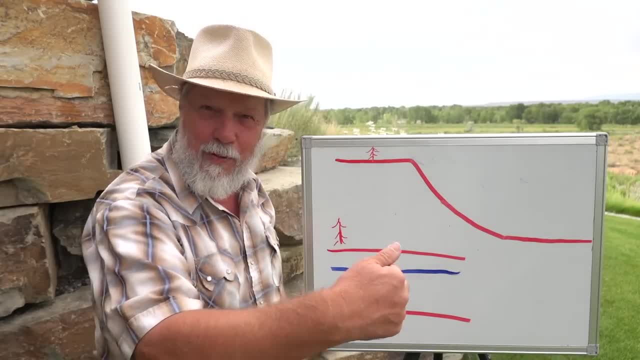 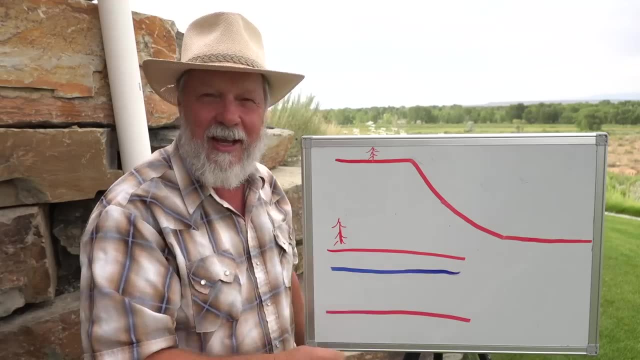 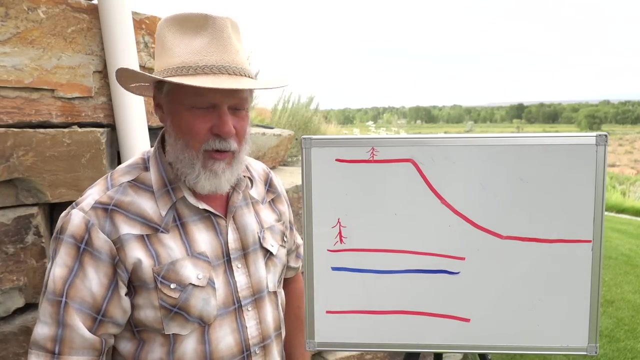 But here it's very stable because there's pressure exerting in all directions. It's kind of like having water in a bucket: The pressure is the same in all directions. sideways. That's a whole lot different than up here in this sketch. So here we have a hillside. 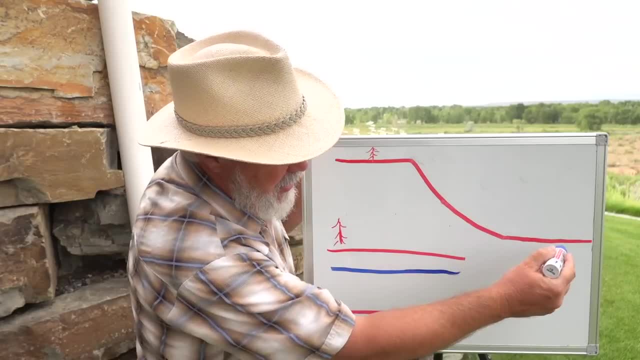 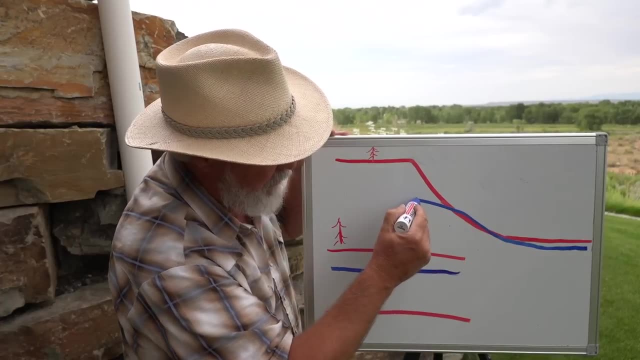 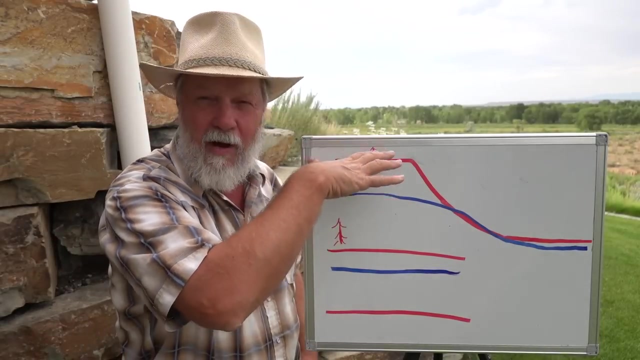 Let me draw in a water table prior to a slide. Let's say it's out here in the flats And as it comes up it kind of intersects the surface and comes out here like so That's fairly common in a hillside if you have a lot of water coming in from rains and things. 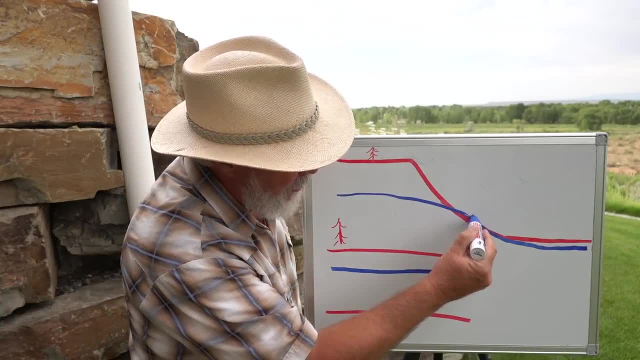 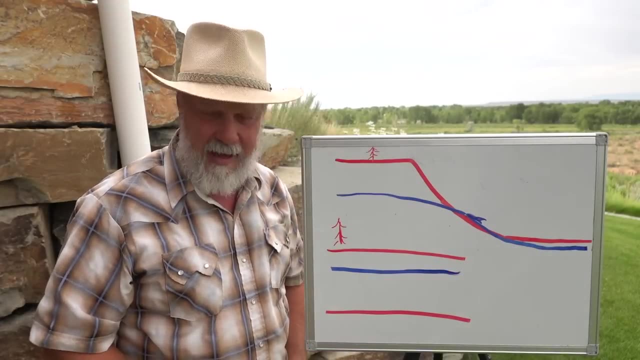 That's kind of the normal, we'll say: And you'll develop a spring right here. You'll develop springs where it intersects the surface, this water table, And in a normal year or normal years, that might be the stable situation here. And this is why it's fairly common to see springs and seeps in areas that are prone to slumping. If you build the water table up- and I'll do that here- a period of lots of rain, and build it up higher and higher, you're creating more and more pressure. 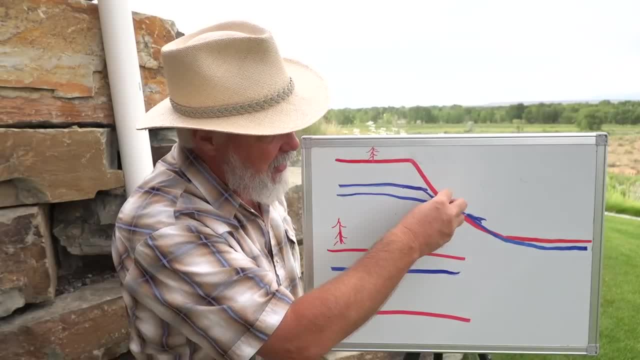 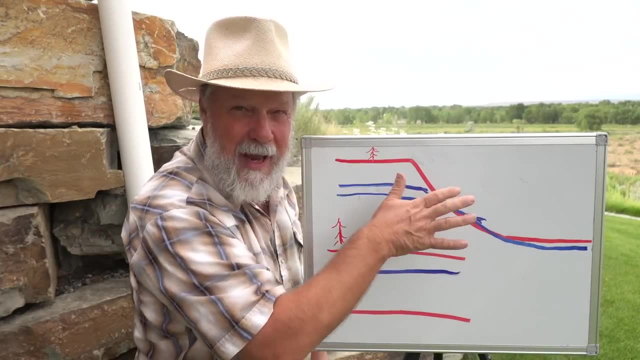 10 feet, 4.3 psi And eventually it is unstable because there's nothing exerting force here. It's like empty space. It'll just blow out the side. It's kind of like that. It doesn't actually blow out, but it's a good mental image. 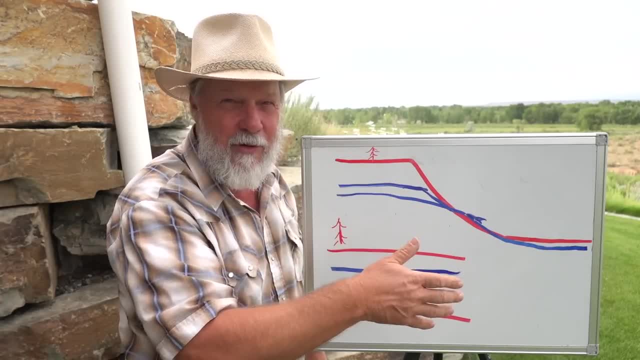 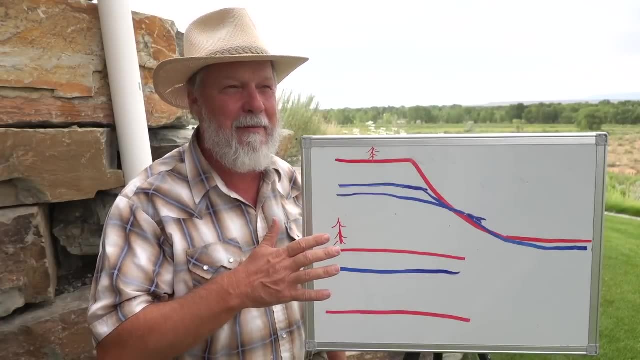 And there you have your landslide debris flows, etc. So this brings up an interesting point, because many people build their homes, maybe in an area that's fairly stable- this earlier case- And what are the first thing they do? They have a home up here. 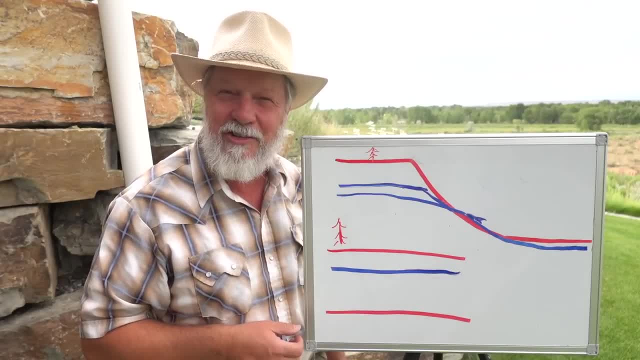 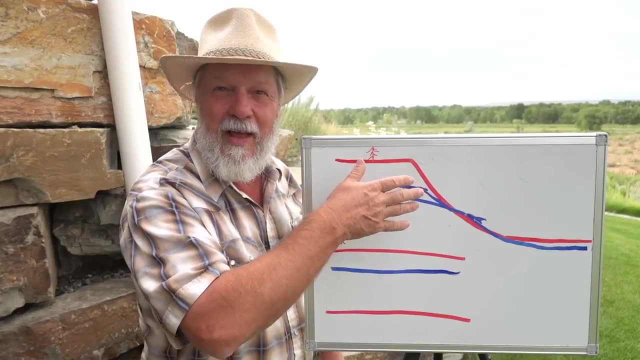 They want to have a big, nice yard And they start adding water to the system. Well, there are many cases where that occurs. They build up the water table. It's unstable, They create a debris flow or landslide and off goes their home. 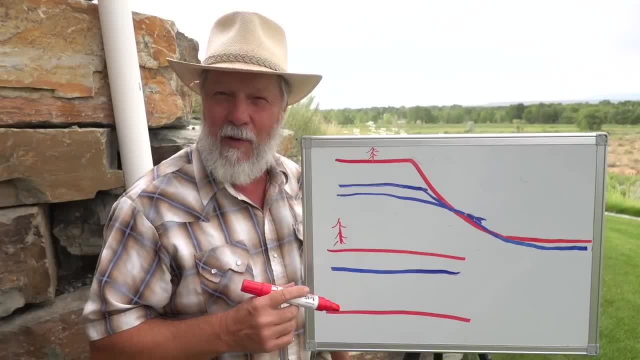 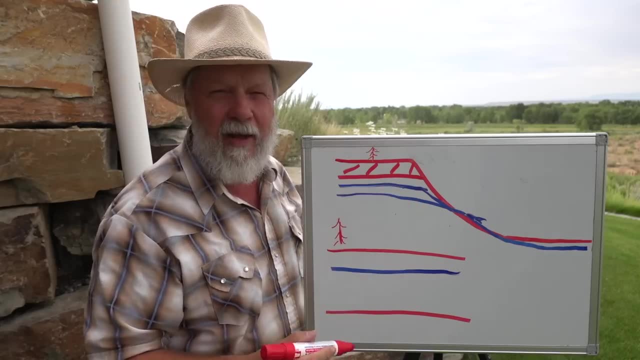 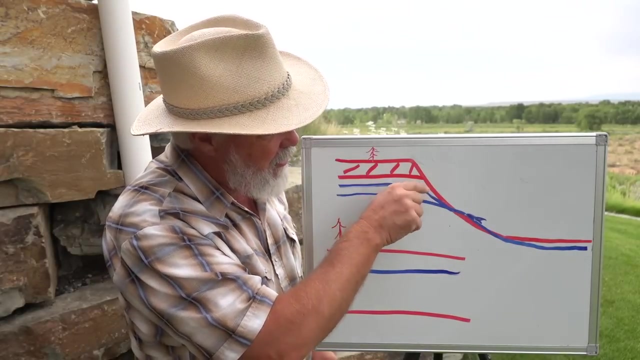 Or worse. Okay. another interesting point I want to make is: oftentimes you'll have- maybe it's really hard- rock up here, Big cliffs of rock- I've seen this- But underneath it are weaker rocks And you build up the water table here. 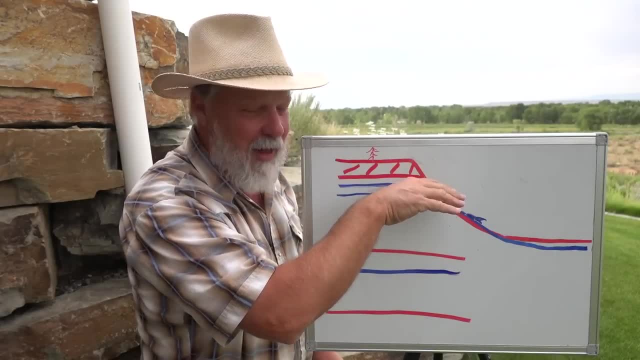 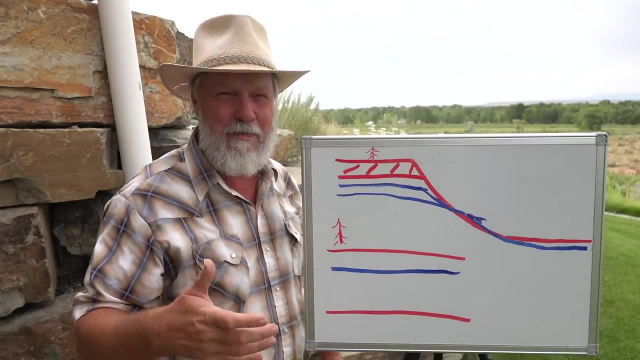 It blows it out off the side, creates a debris flow, landslide, And, of course, if you're removing material here, this is very unstable. And now you have these big rock avalanches right along with it, And that's not so uncommon either. 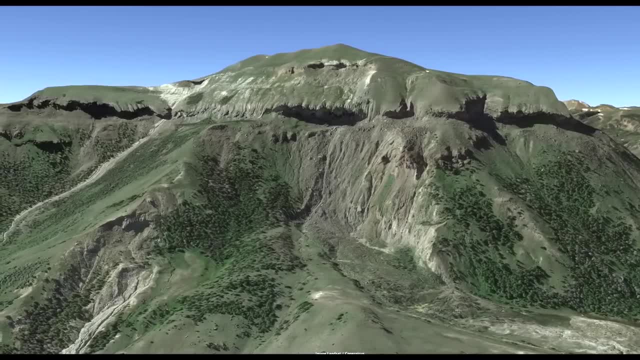 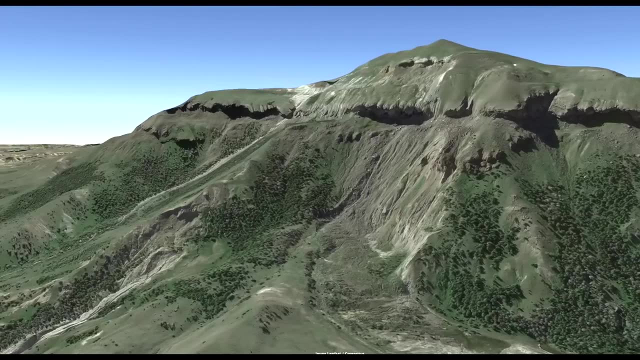 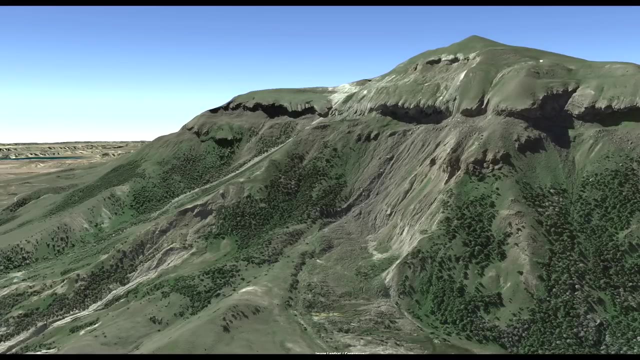 Here is an example of what I was talking about. The massive cliff that is broken away here came down on the debris flow below. The contact between the mudstone and the volcanics above it is about here. Let's zoom out and take a look at this huge debris flow. 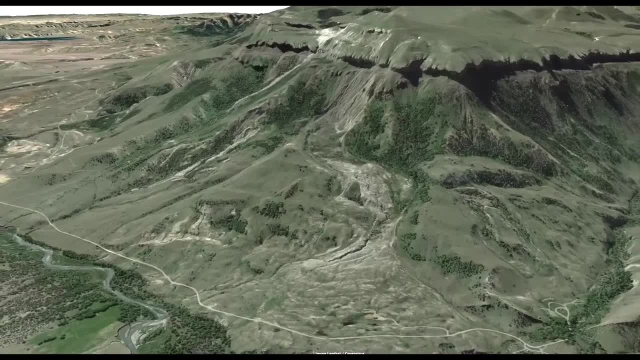 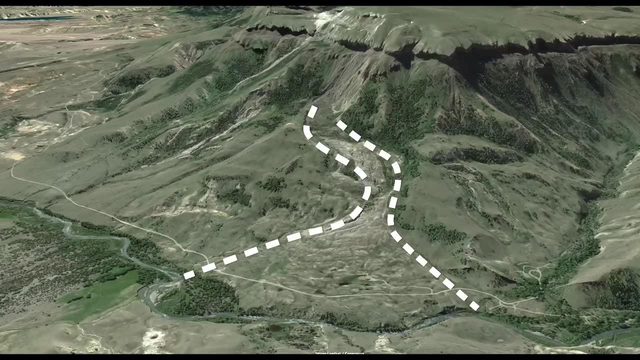 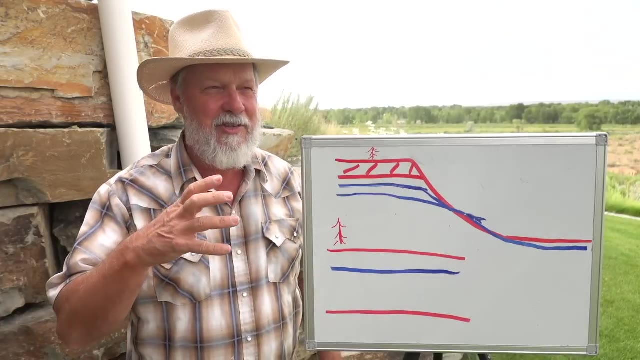 Wow, it's really quite impressive, isn't it? Notice the buildings here. This is a pretty old one, but the features are easy to see. Our knowledge base is now where it needs to be for the most important part, Because we understand reasonably well the modern ones and their features. 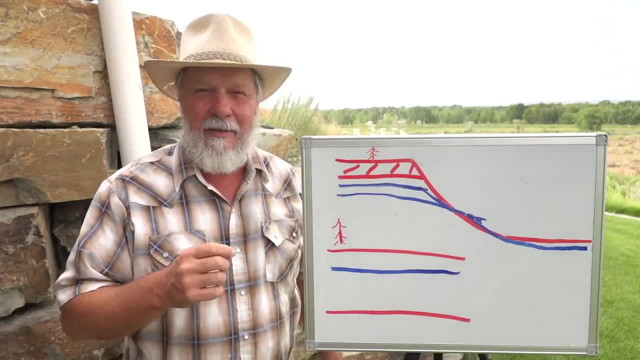 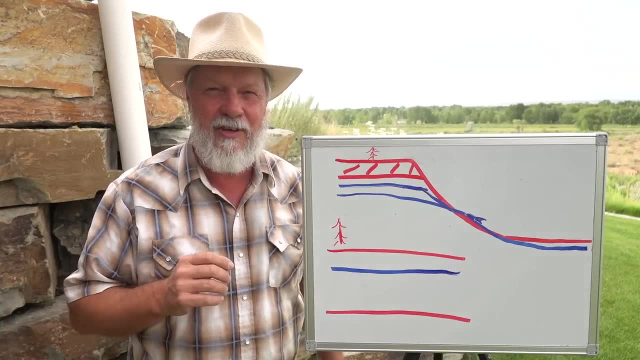 and how they form and why they form, But we need to be able to recognize the ancient landslides, As I've mentioned. that's where the danger is going to be Whenever I see a modern one occur. I know that almost always. 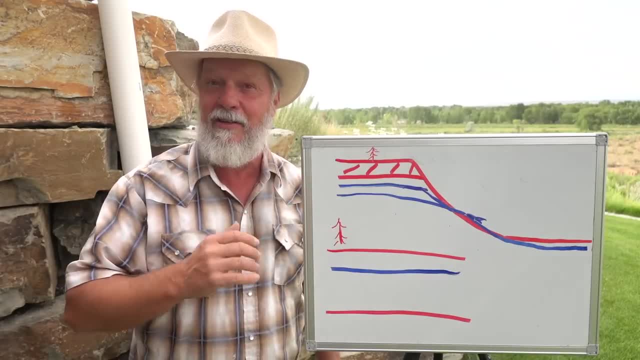 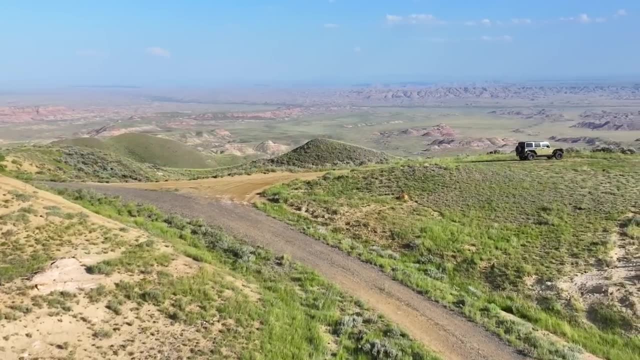 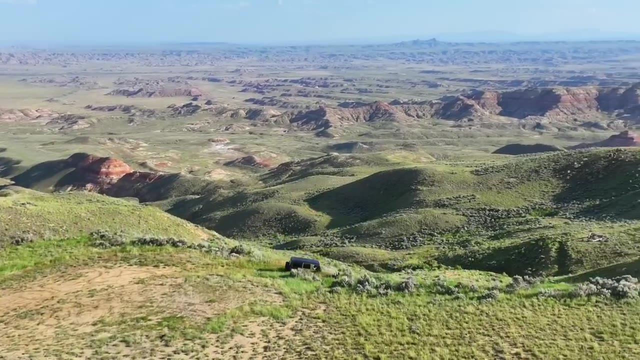 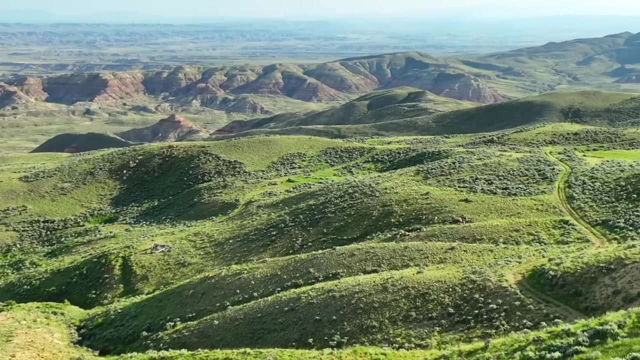 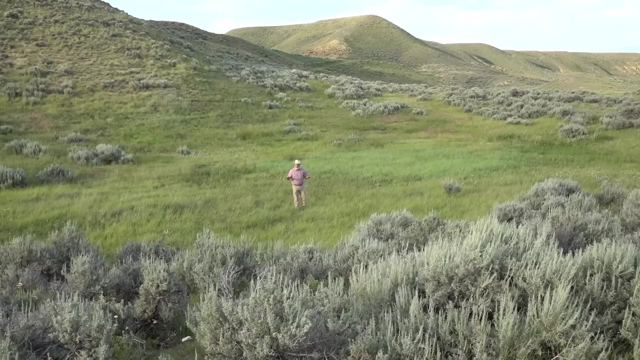 we're going to have ancient ones that occurred prior to that. Now that we've seen modern examples of landslides, let's start to unlock the secrets of ancient landslides and learn to recognize them, even when the clues are subtle. I'm standing in a feature that is an important clue. 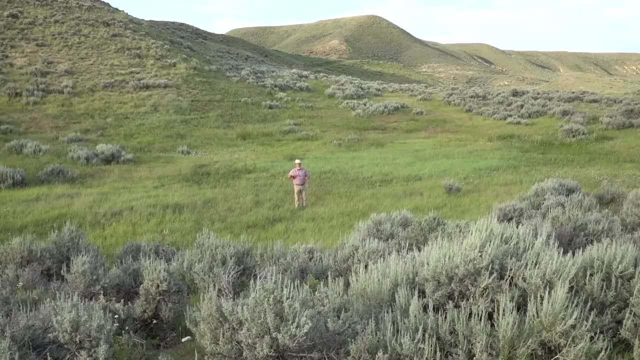 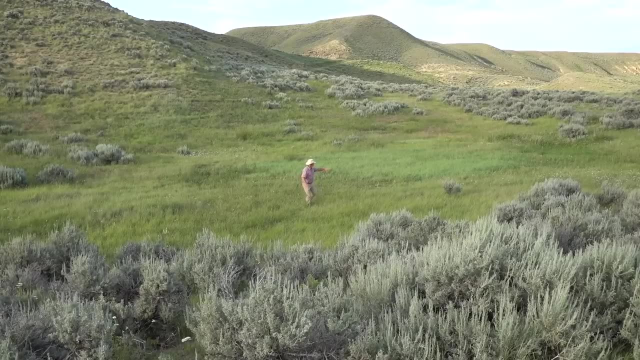 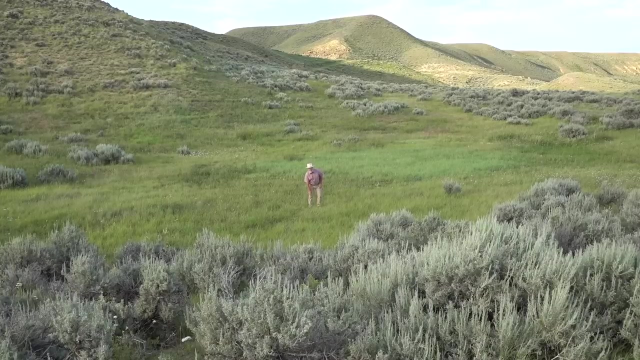 to mass wasting or slumping or these landslides with rotational blocks. And that is this low area. This nice grassy area is low. If you had a lot of water come in on a heavy rain it would probably get almost up to my knees deep. 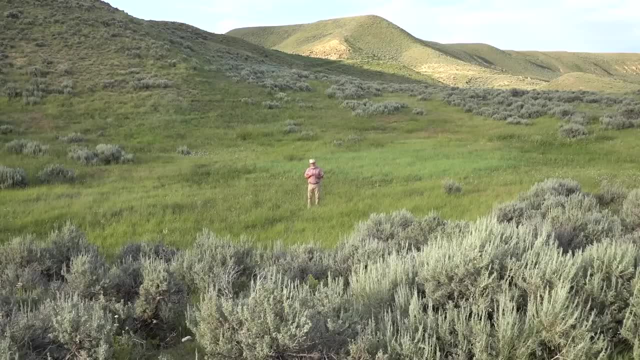 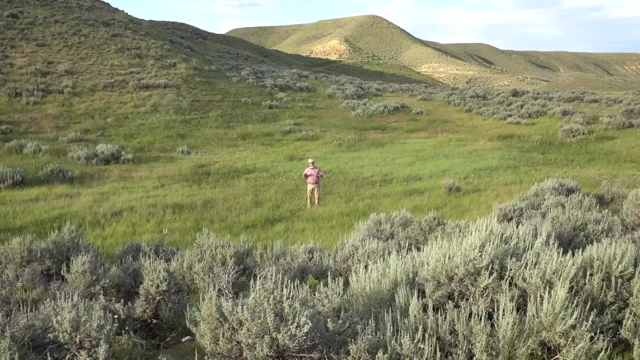 And it turns out to create lakes and ponds is very difficult to do unless you have glaciers involved. So really, the vast majority of ponds and lakes and low closed areas like that are from glaciers. However, there's another process. that's the second most common. 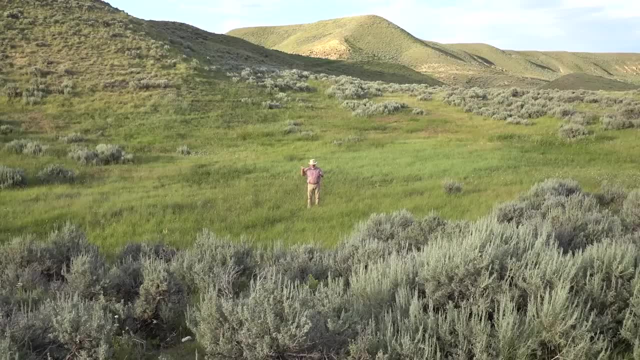 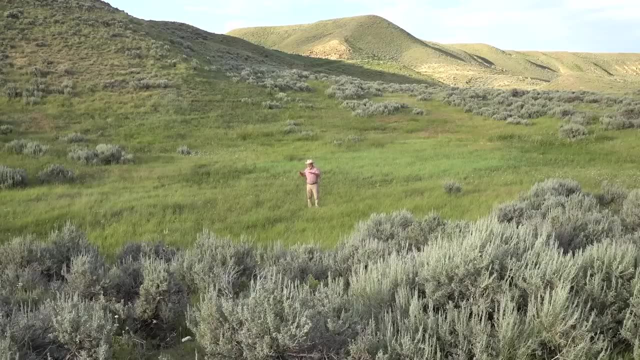 If you're away from glaciers, it's landslides and slumping where you rotate these blocks and get low areas like this one. We're going to look at this with the drone and then tie it into the bigger picture and see what's going on. 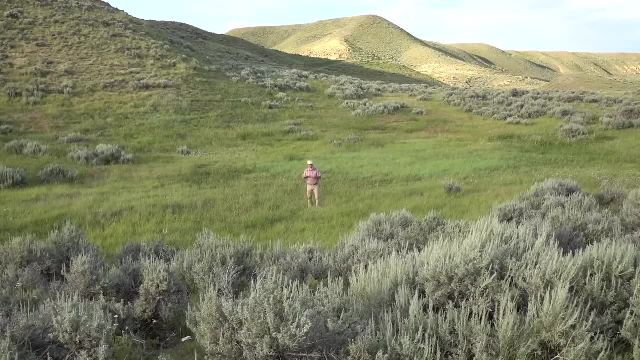 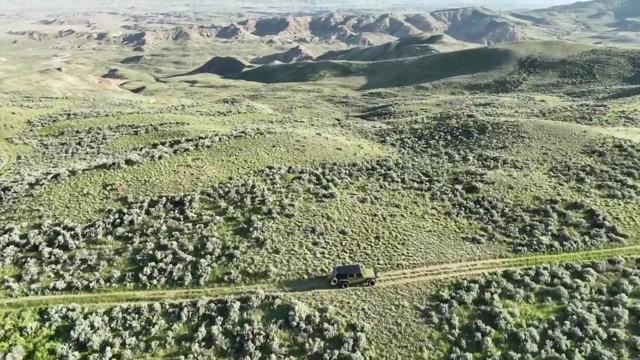 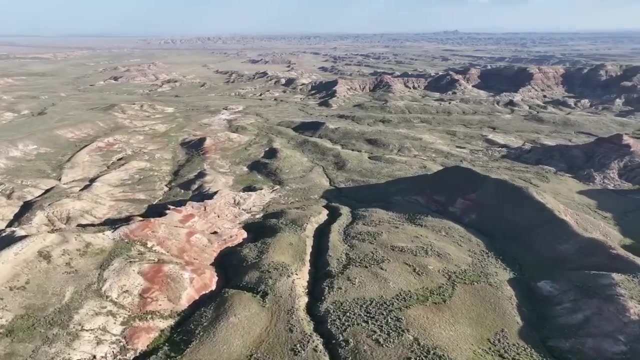 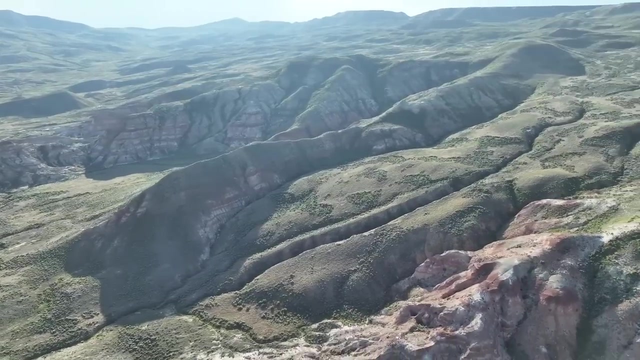 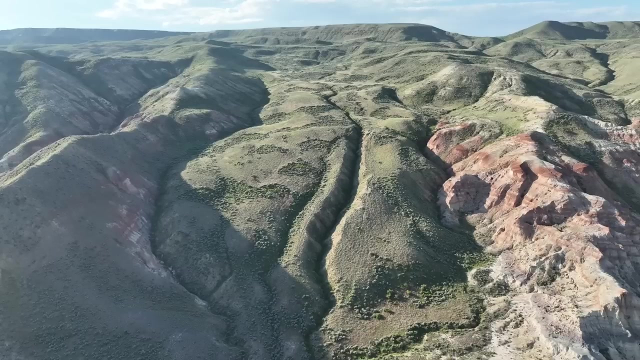 and see how this gave us clues to what is happening out here. This incredible debris flow is becoming more and more obvious as we fly down to the toe. Zooming in, we can see just how ominous it is. It's about 650 feet wide, over a half a mile long. 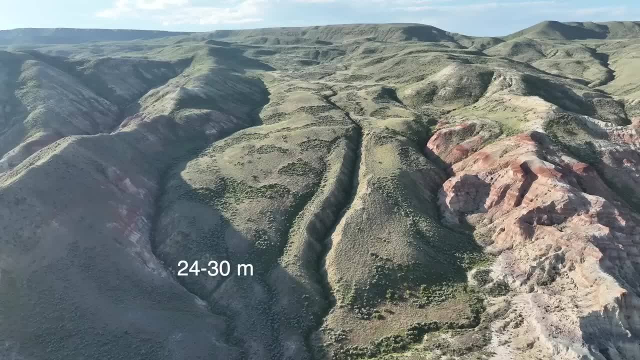 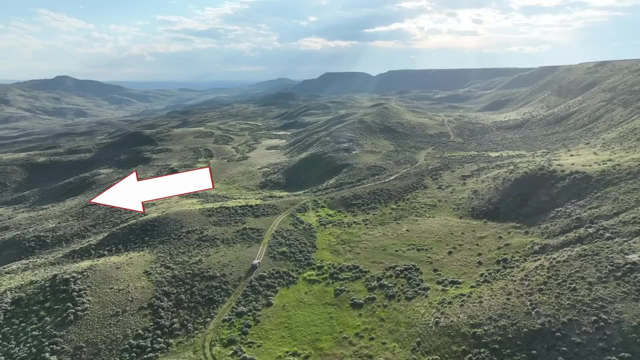 and 80 to 100 feet thick. It came down a pre-existing canyon with sides we see in the red rock on the right and on the left side. Now let's look in another direction, from high above the low area. The debris flow we just viewed is down the mountain to the left, out of view. 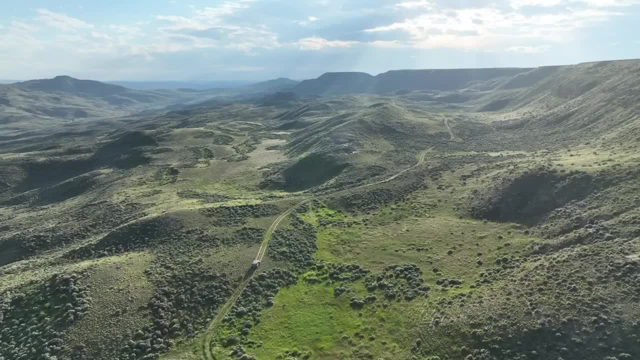 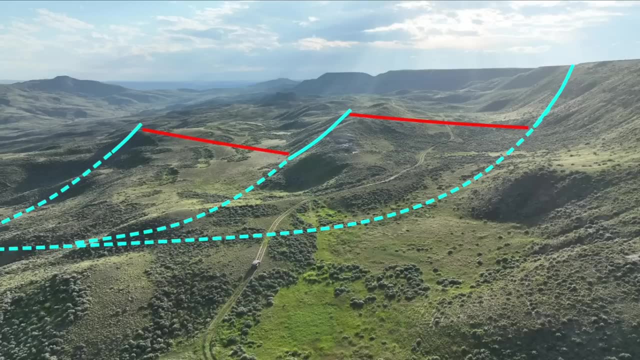 When I view this scene, I draw a geologic cross section in my mind. Let me show you what I mean. I visualize three faults forming scarps with two benches marked in red. The dashed part of the blue faults is what is underground. 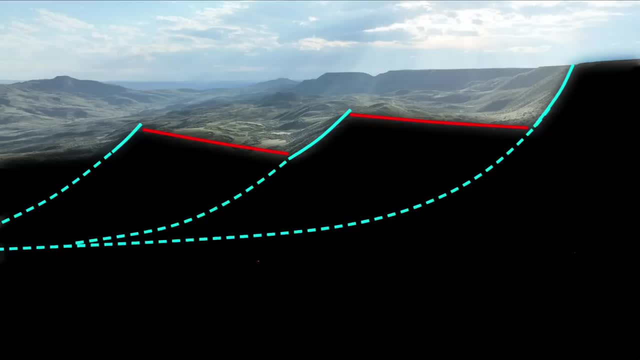 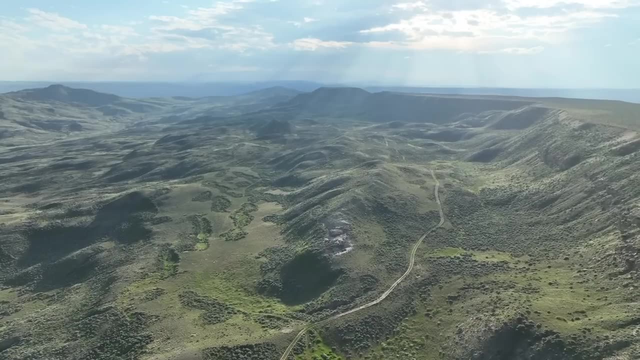 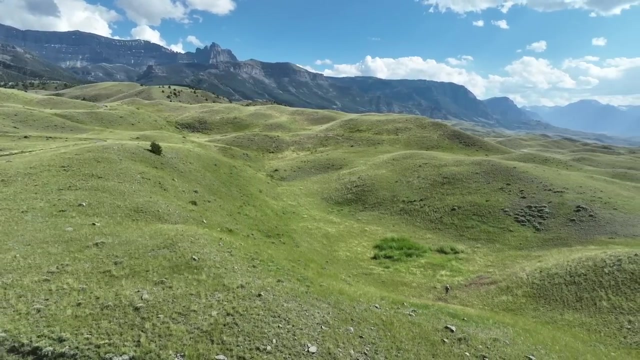 Here I've blacked out the area that is underground to help you further visualize the scene. along with me- Isn't this fun? As I walk down into quite a large low area, I try to visualize the great events that have occurred here. 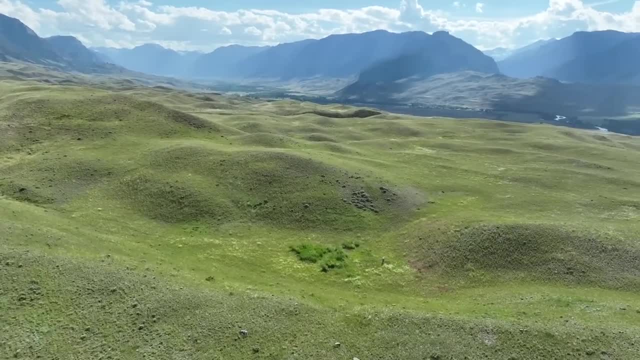 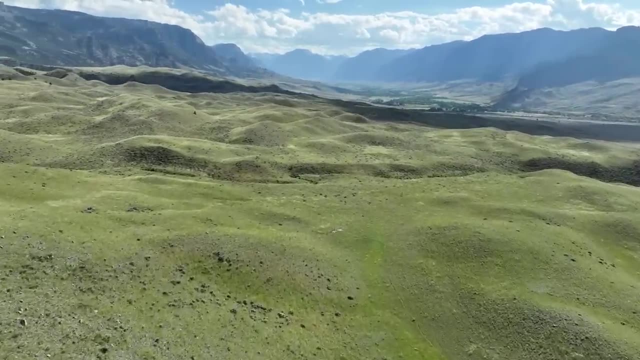 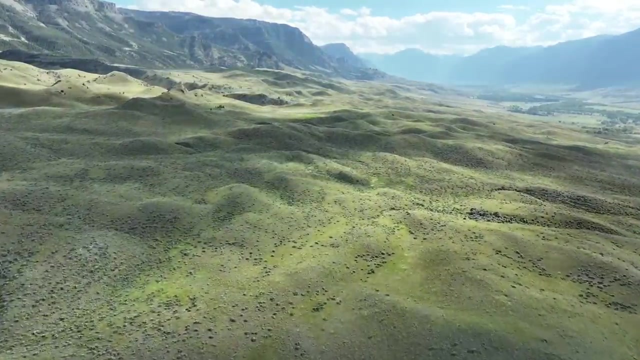 Here I can see a vast terrain of hummocky rolling hills mixed in with low areas. From above, you can see a vast terrain of hummocky rolling hills mixed in with low areas. Could it be that this entire area is a massive landslide field made of slumps? 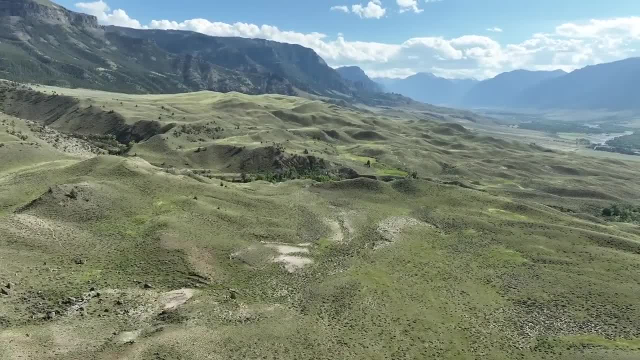 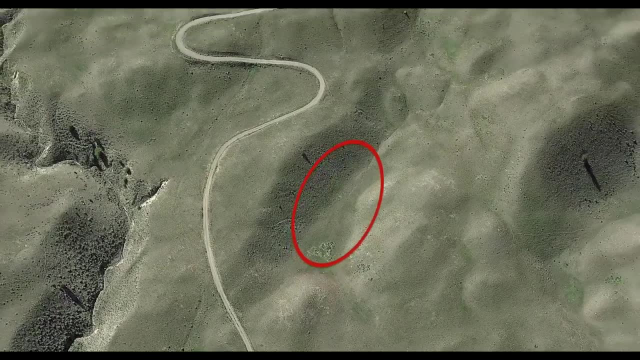 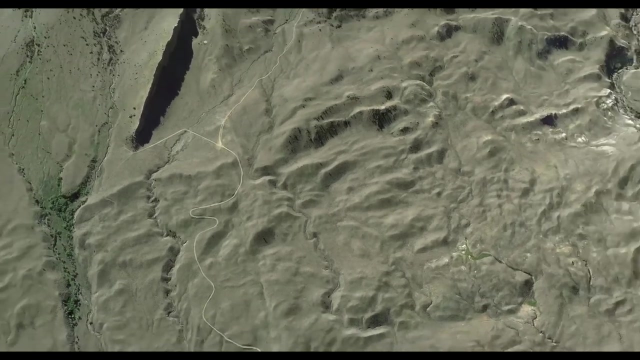 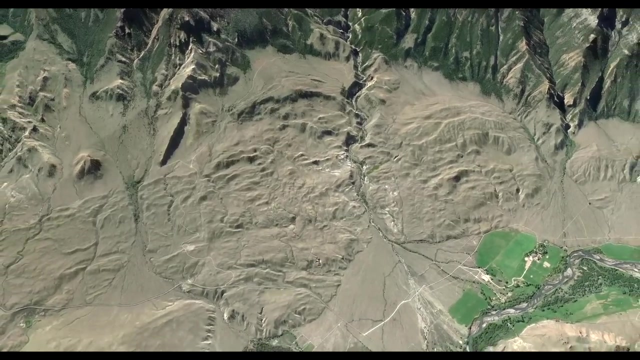 Let's see what we think from a Google Earth perspective. Here is the low area I was walking in. Sometimes we need a larger perspective to understand a geologic setting, and this is a case in point. I see two massive landslide complexes here and here. 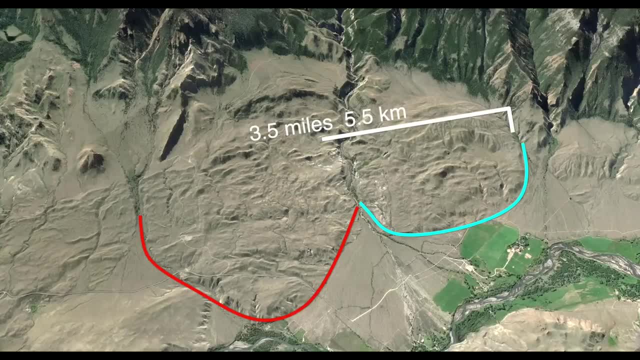 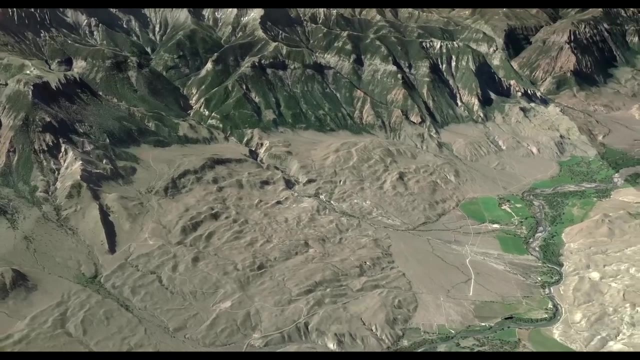 The distance across them is about three and a half miles, and they are 100 to 200 feet thick. Boy, this is really hard to get your head around, isn't it? Looking closer, we can see a few more details. All up and down this valley are similar landslide complexes. 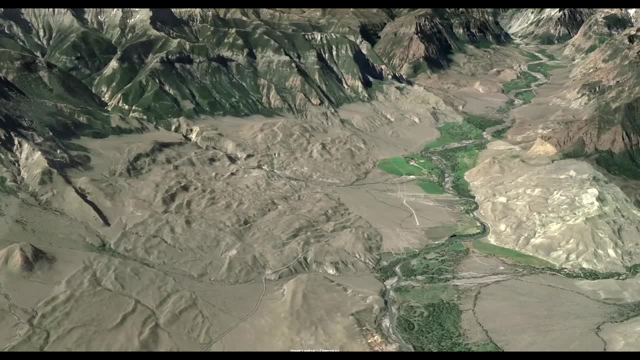 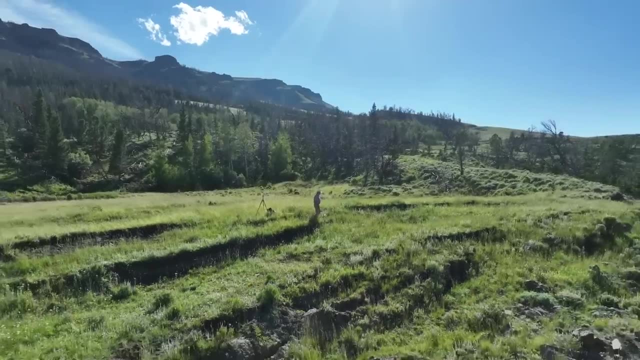 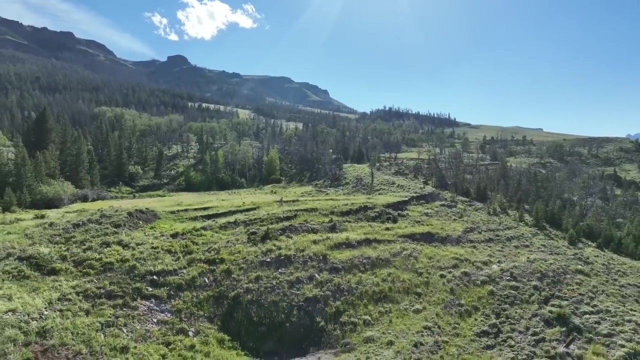 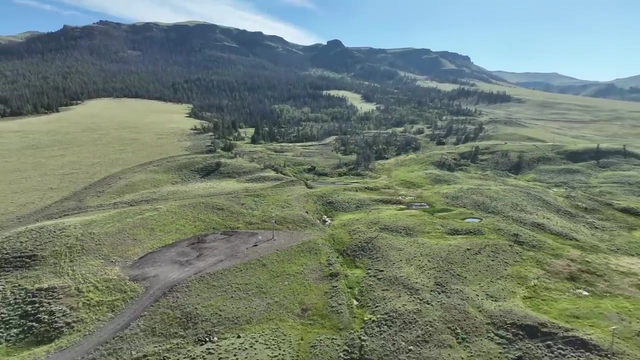 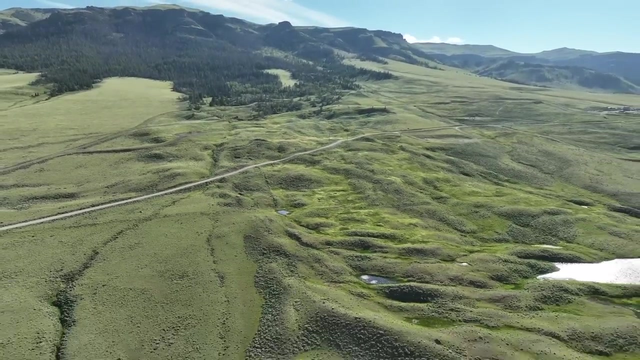 Believe it or not. in a nearby valley there are many homes built on similar complexes. Well, we see some minor breaks in the Earth's surface here, forming these series of small benches. Let's see what it leads to. I hope you're seeing the boundaries of a massive debris flow. 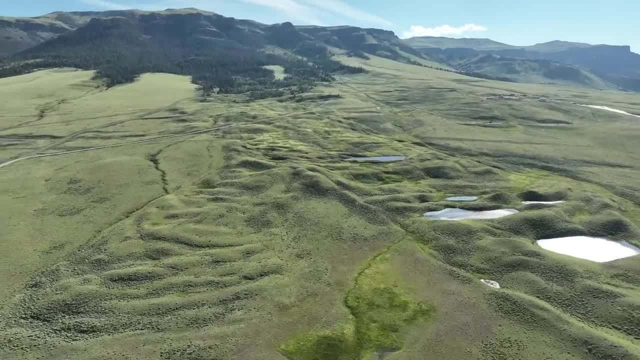 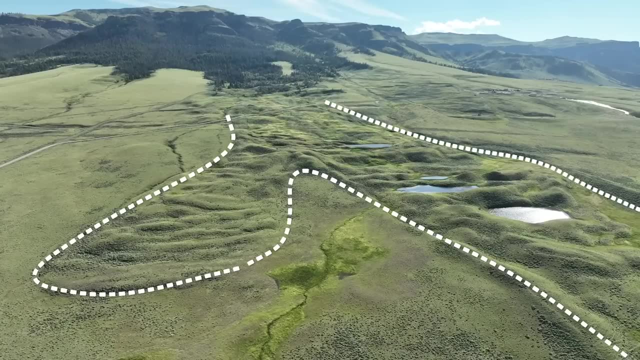 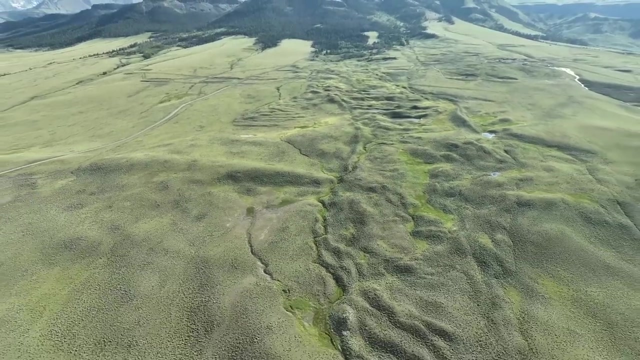 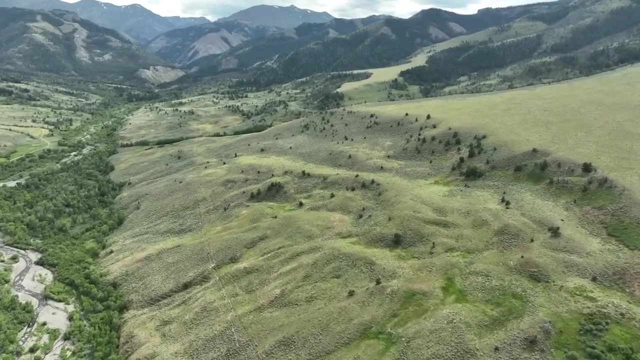 All of these ponds are definitely a clue, aren't they? I see a debris flow that divided into two pathways in this area. Let's continue. The run-out on this landslide is some two miles or three kilometers. Here we see nice bite-shaped scarps with much slumping below. 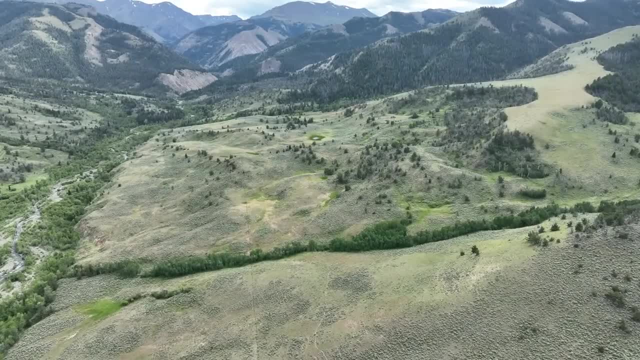 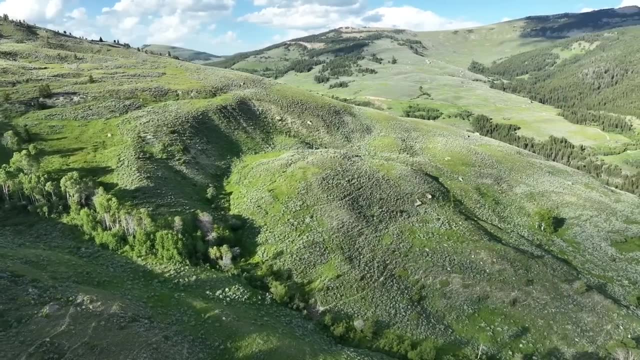 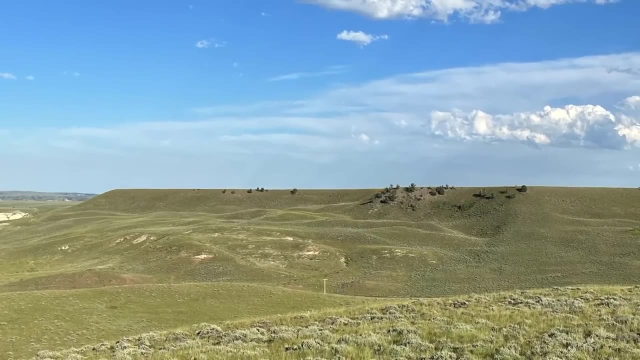 It's quite easy to identify the scarp and the slump in this old landslide, But in another case, this one isn't so obvious, is it? What do you think of this terrain? It sure has a hummocky look to it, doesn't it? 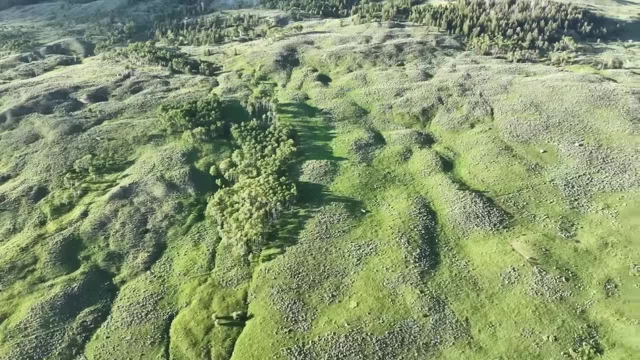 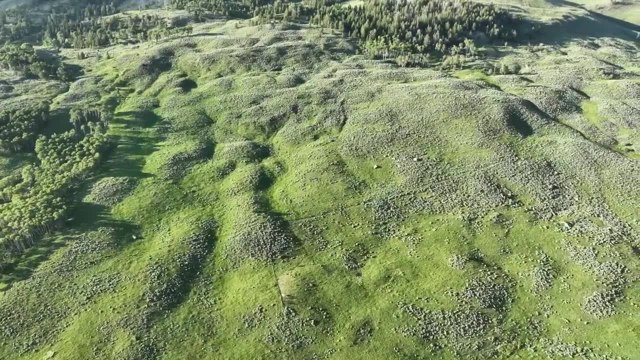 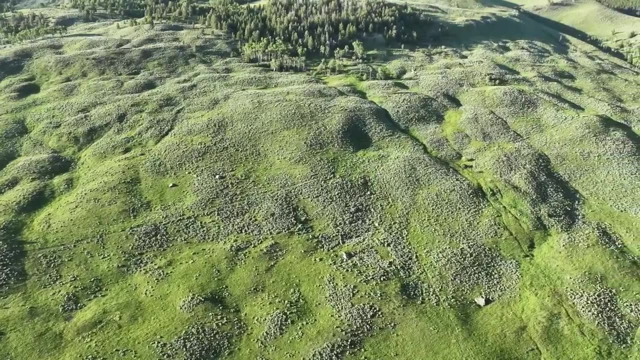 Some might would say rolling hills. The whole mountainside is a mix of slumping and debris flows. It can be very helpful to know the name of the sedimentary or rock layer that shows evidence for landslides. By knowing this information, you can correlate and or identify the layer. 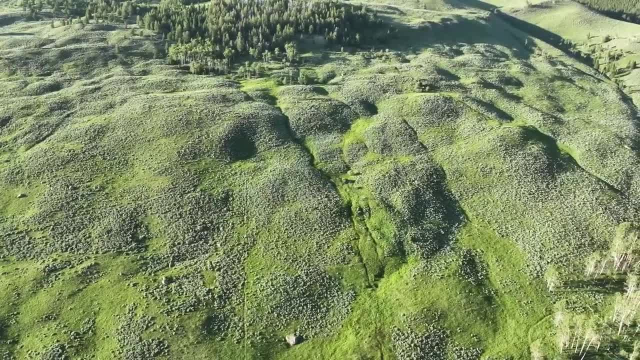 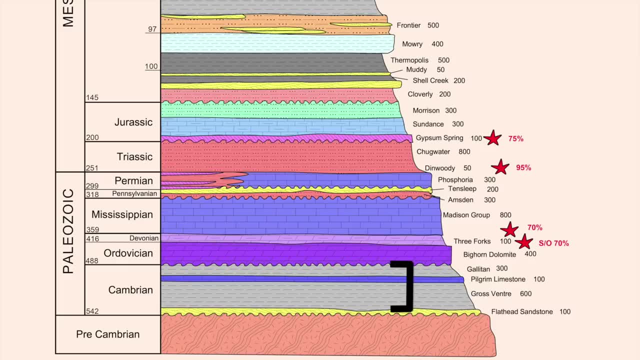 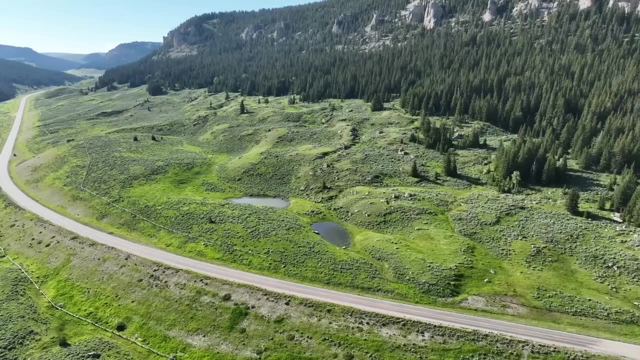 over large areas and pay particular attention to it. The sequence we've been observing is shown here in this stratigraphic chart showing the rock layers. It is some 1,000 feet thick and is dominated by shales. Here is another view of this sequence: about 30 miles from the prior area we viewed 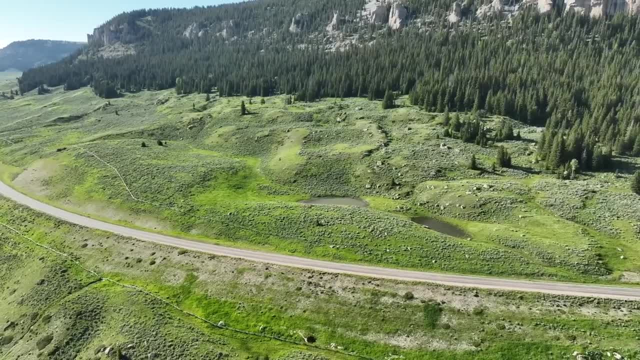 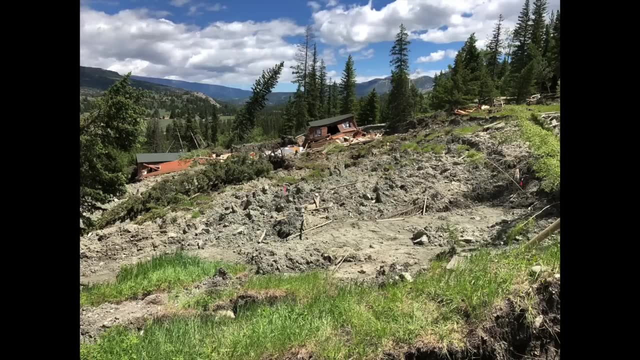 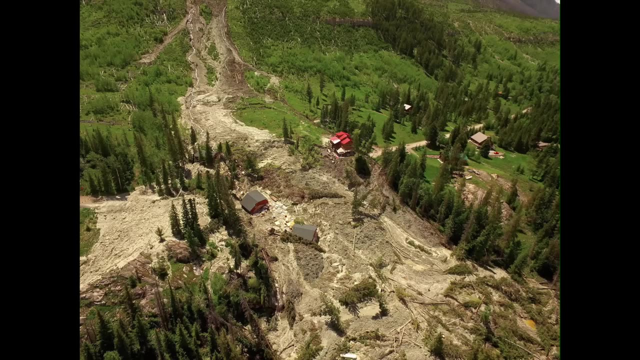 It sure looks similar. Notice the ponds. Following this sequence, 100 miles across the basin, we see that it is prone to slides, where several homes were destroyed. This looks familiar, doesn't it? But let's see what we see adjacent to this debris flow. 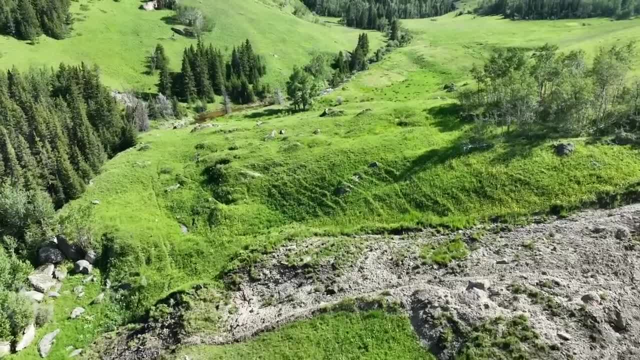 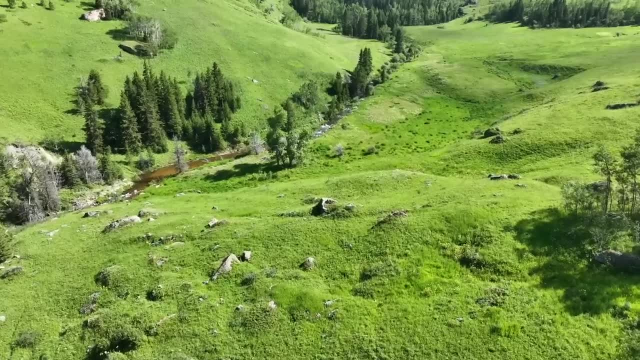 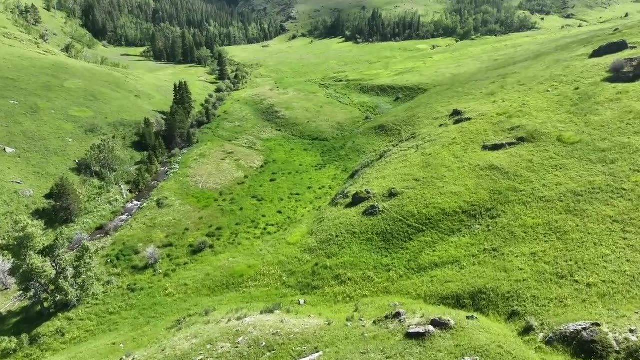 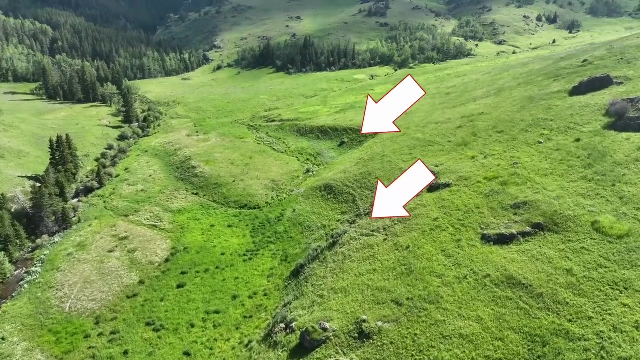 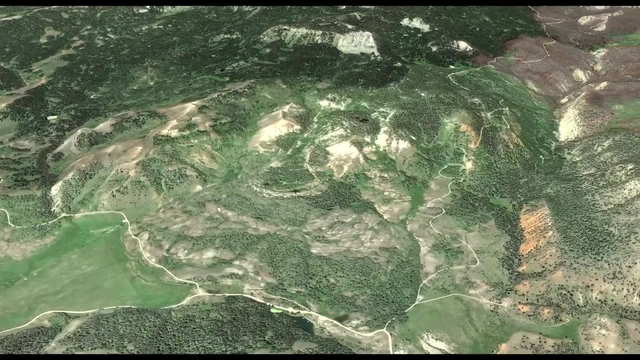 What about this area here? I think it's the bulging toe of an ancient debris flow, with large boulders on top of it. Continuing further, I see two bite-shaped scars from small slumps. This spectacular debris flow would be difficult to identify. 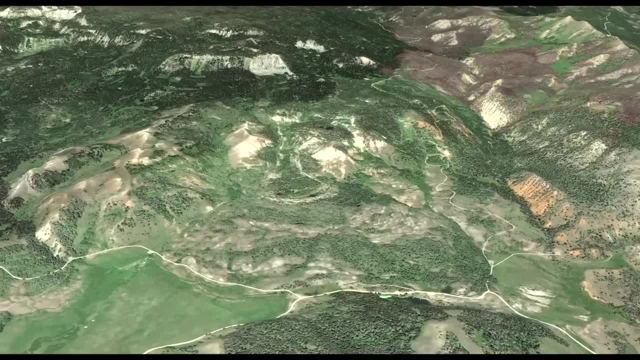 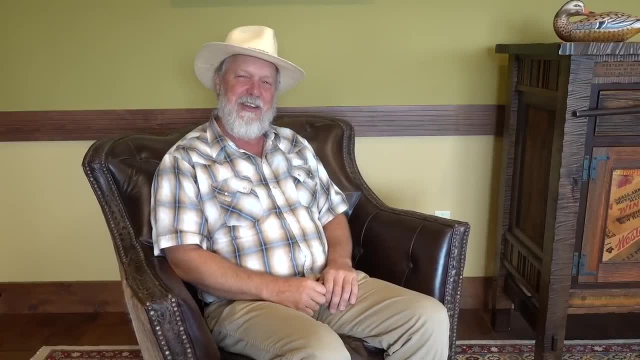 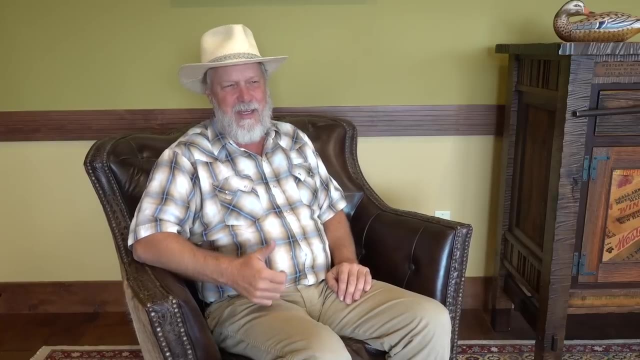 without the aid of Google Earth. The headscarp is way up here. Are you ready to have some fun? You're going to be the geologist that evaluates a few areas for potential landslide risk. This would be great practice for you in your own situation. 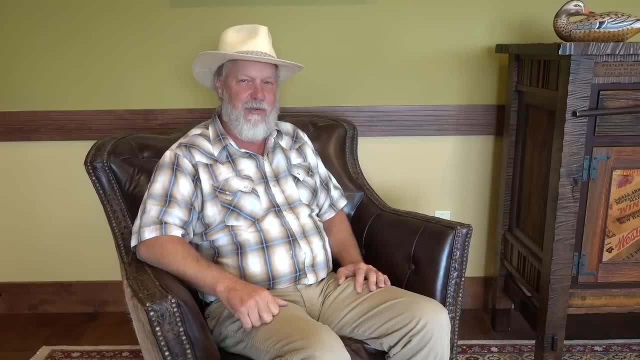 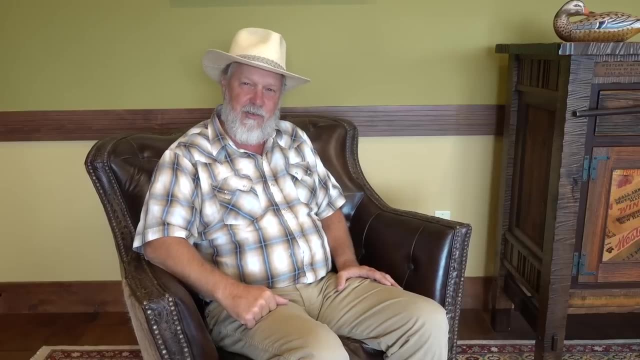 Now, not to worry, you can always have a geologist look at your property. I know one well that could help you out, and I've included his contact information in the description to this video. So let's get started looking at these areas. 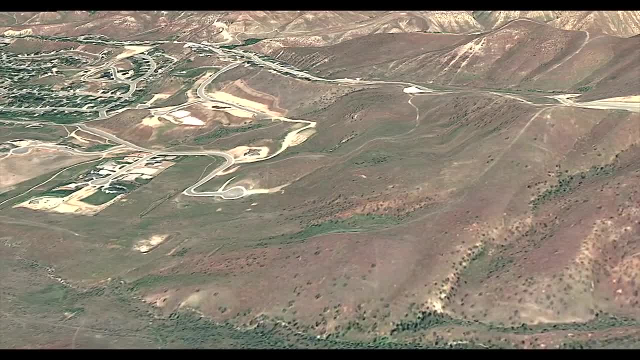 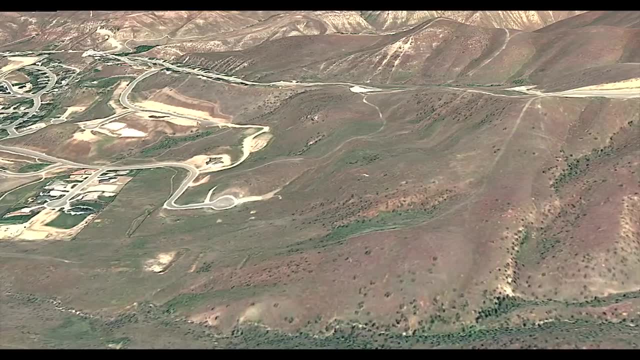 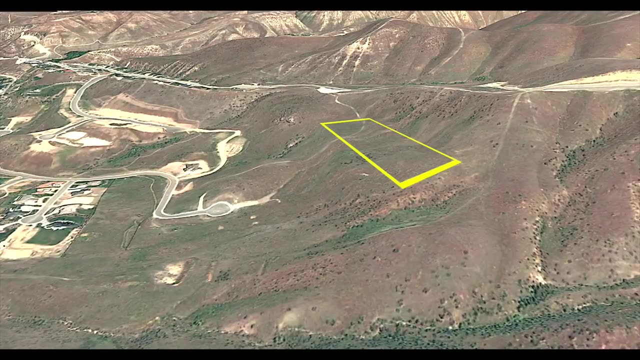 Well, here we go. You're the geologist. What do you think about this potential area in Idaho as a development? Are there any hints of old landslides that you can see here? A developer is proposing to place homes here. What do you think? 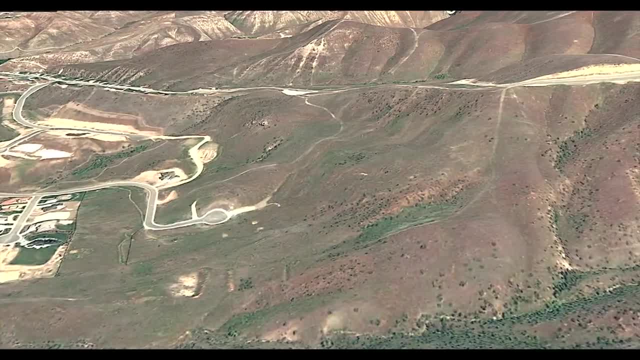 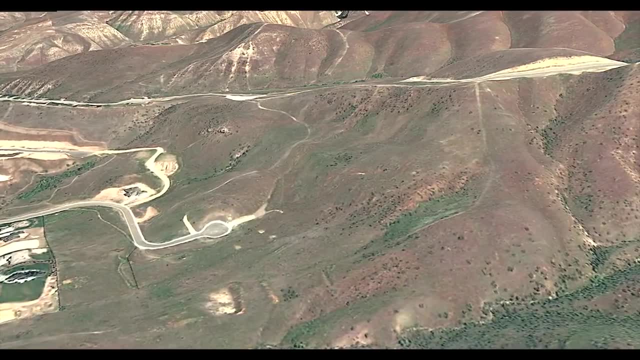 I'll point out just a few of the features that I see. How about this nice headscarp along here, And right below it, as you might expect, is a nice flat bench, which of course makes a nice area to put homes on, doesn't it? 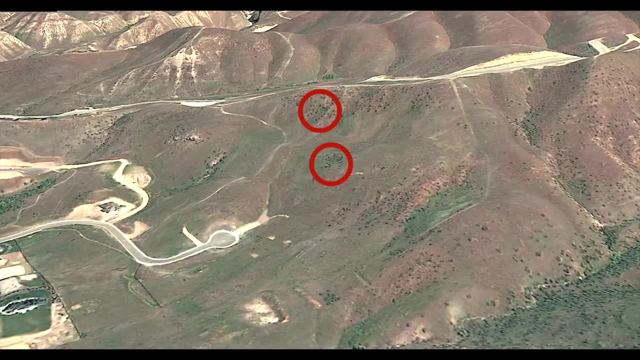 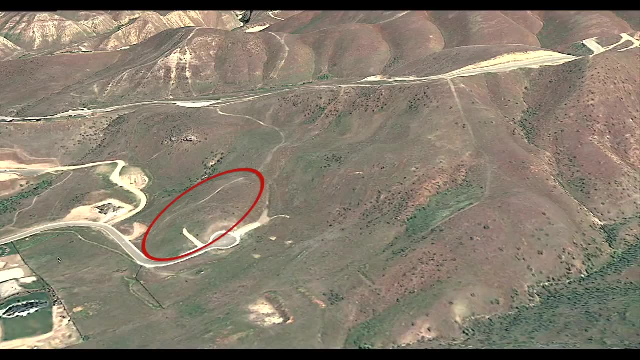 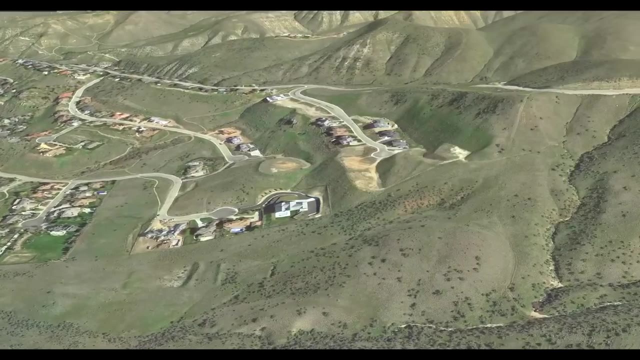 I see green areas that suggest water weeping out through the rock, And also I see a very nice slump feature right here. Thanks to Google Earth, we can go through time and see what happens. Homes were built along the bench we were talking about, right below the headscarp. 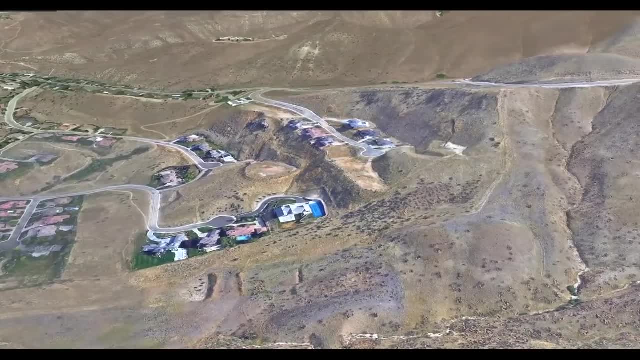 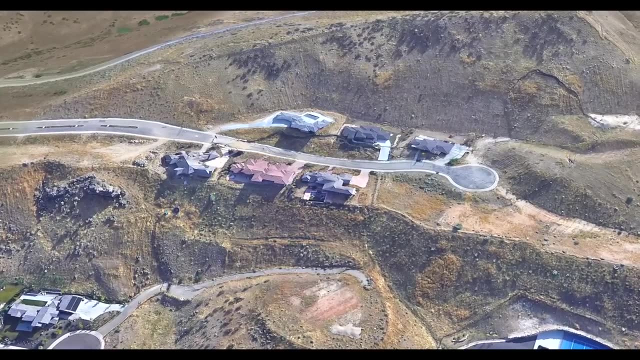 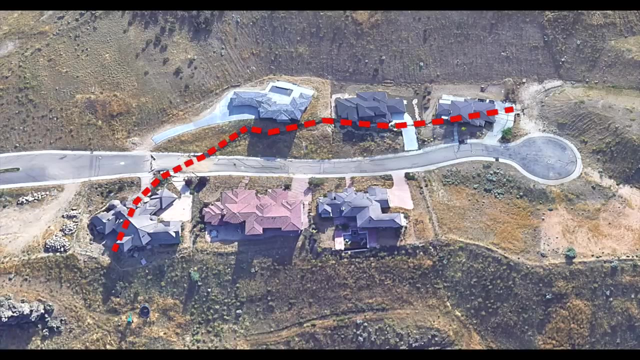 But this image a year later shows that major problems have developed. Let's zoom in and take a look. The structure that developed certainly caused a big problem with these homes. It seems that California is in the news all the time about landslides. 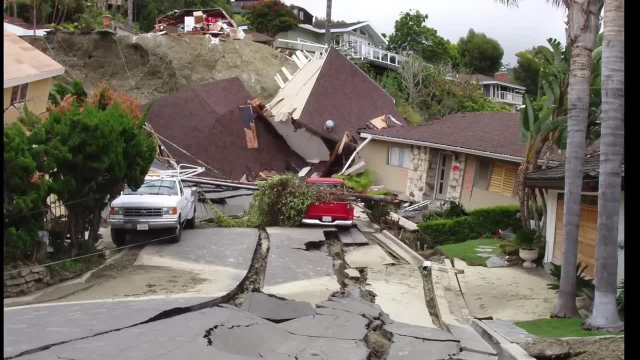 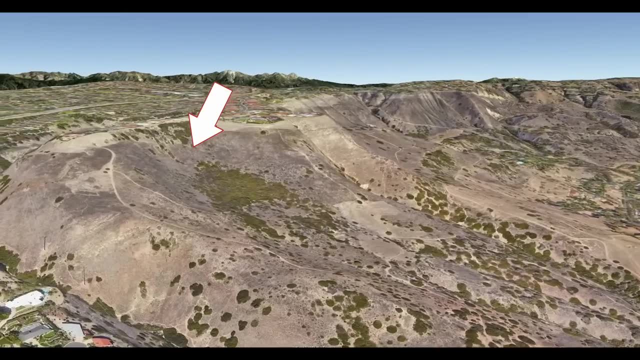 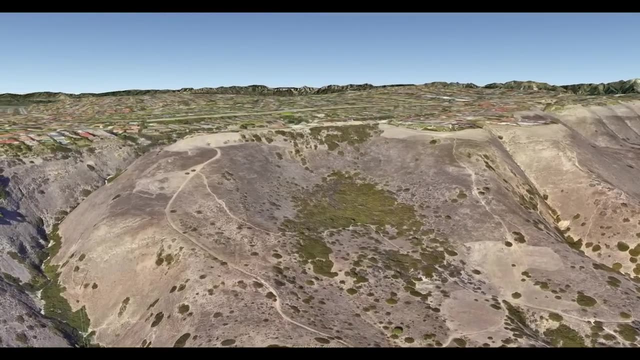 Let's review just two areas to see what you think. I see an ancient headscarp here that has the classical bite shape to it. Also, note the greener vegetation here. It's kind of difficult to see, but there's a whole row of homes. 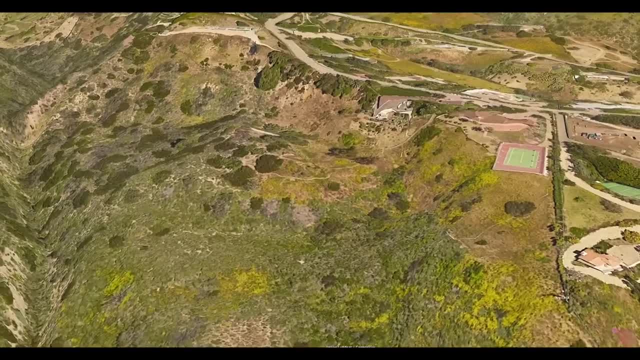 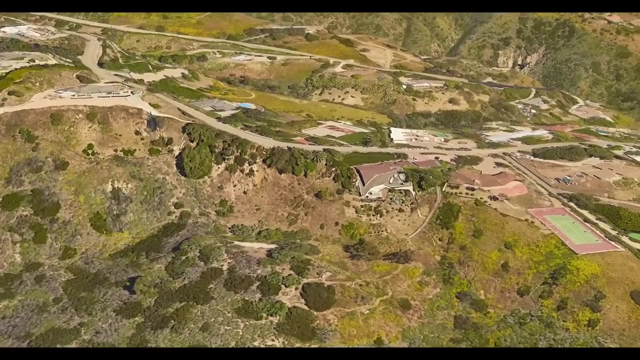 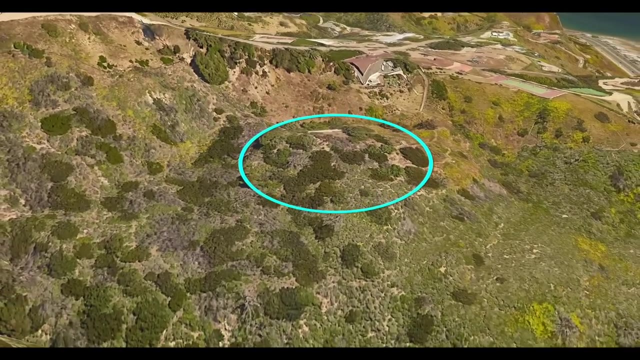 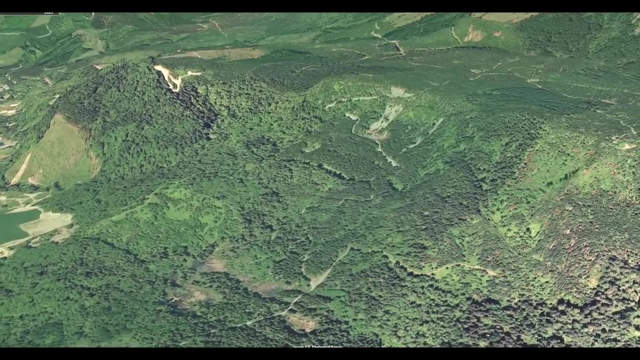 at the top of the headscarp. here, In a different area of California, again, it looks as though these homes are built along the top of a headscarp. Here we see a nice mounded slump feature Moving along. let's go to another state where the terrain is heavily forested. 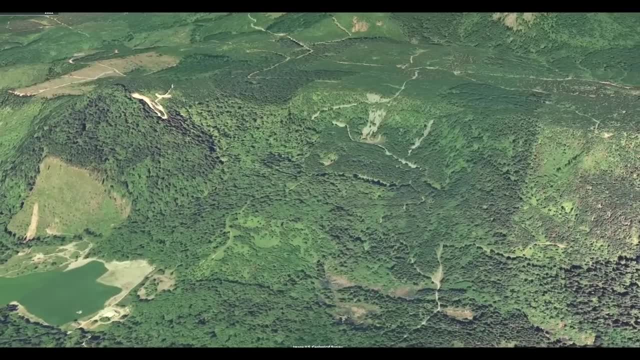 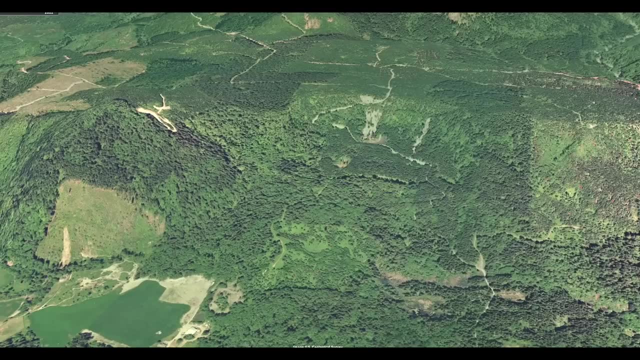 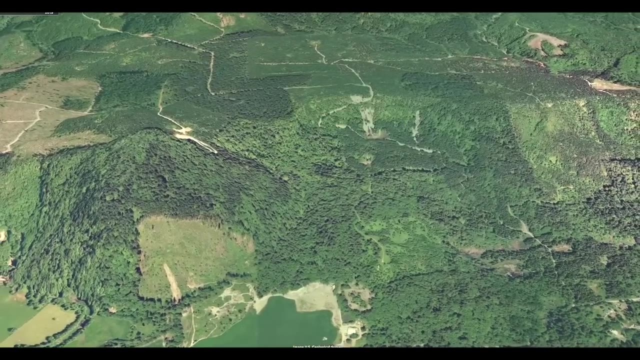 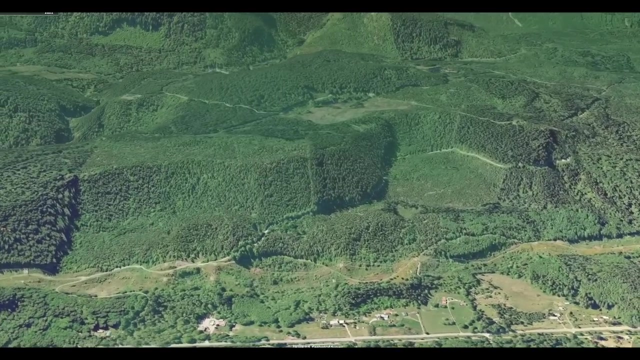 This will be more challenging because the trees can hide details. I see a bite-shaped headscarp- a mounded slump feature here, and it looks like two small landslides here and here. This one's pretty easy. here, Two bite-shaped headscarps with flat benches below. 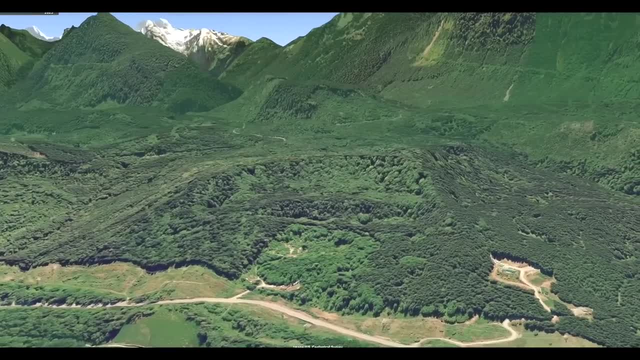 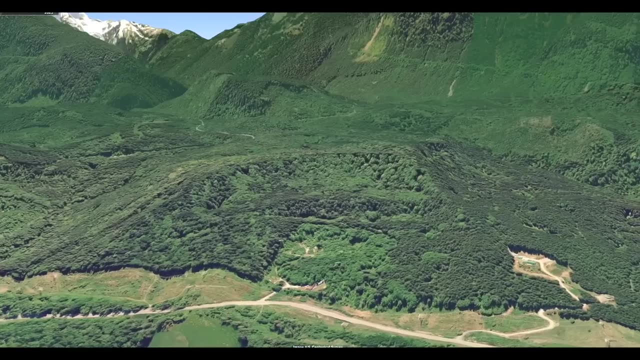 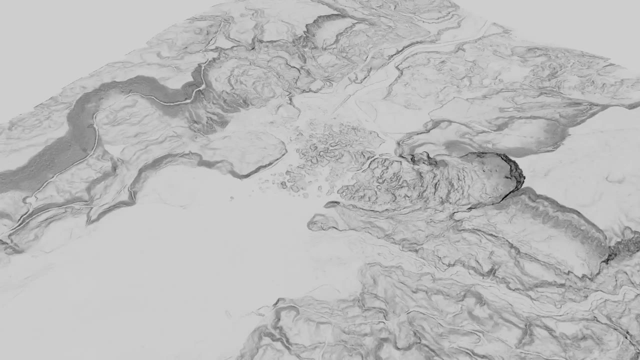 There are certainly some classical features here we can see. in this location I see a main headscarp and then two smaller headscarps below it. LiDAR is a technology that uses pulsed lasers to very precisely map the surface of the Earth. 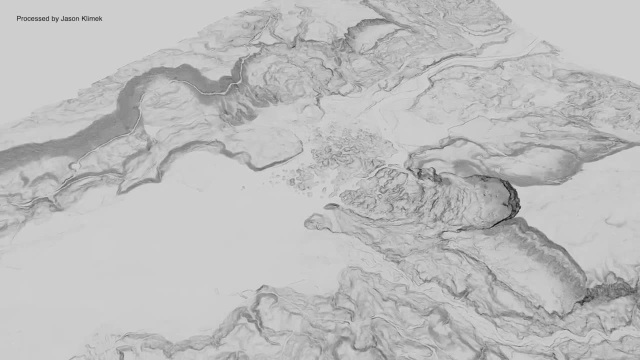 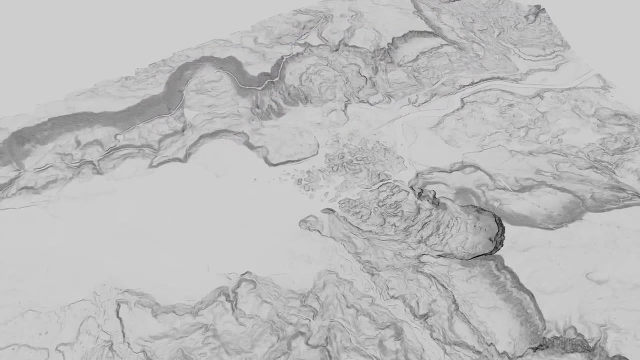 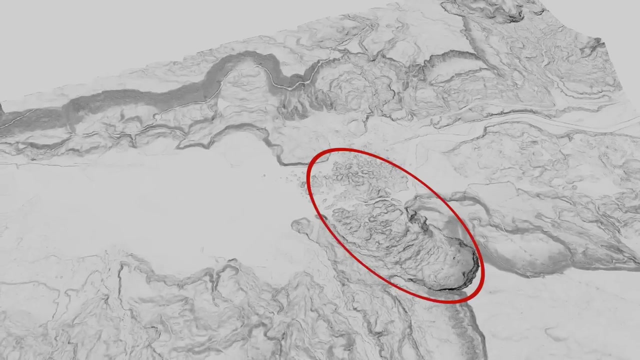 and can be used to remove the vegetation and reveal all the details. Three of the features we just reviewed are shown here. They look quite obvious now, don't they? There is evidence of several other slides scattered about in this dataset, but none so obvious as this one. 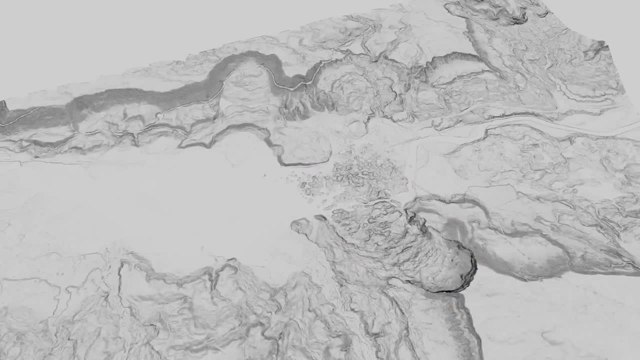 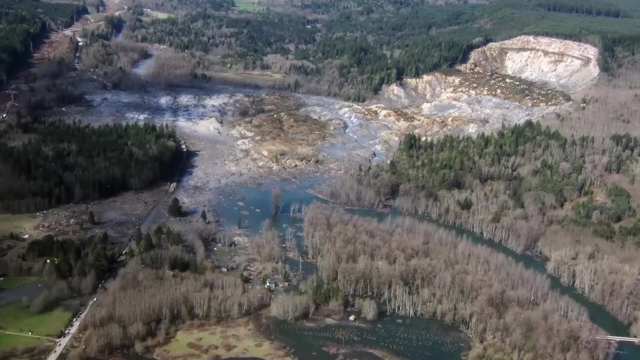 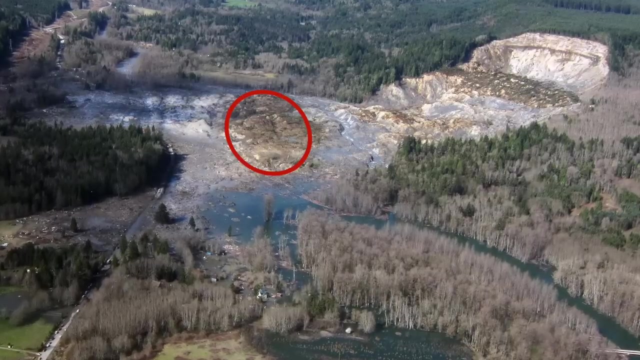 It is the infamous 2014 Oso Washington landslide that killed 43 people and destroyed 49 homes and structures. This landslide fluidized into a massive debris flow with much destructive power at the toe of it. Most of the destruction occurred in this area. 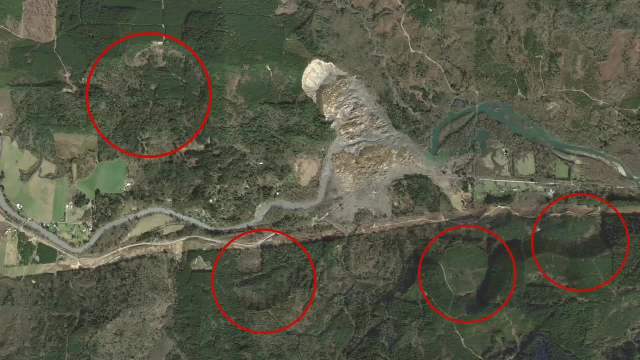 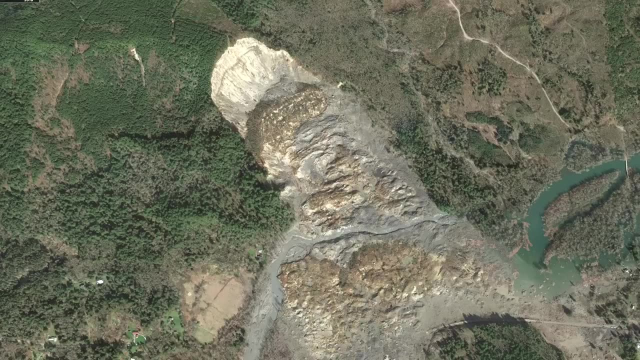 Here we see all four of the forested old landslide scars that we evaluated adjacent to the Oso slide. Using Google Earth, we can review the Oso slide area before it happened and progress through time. I have outlined the core of the slide in red. 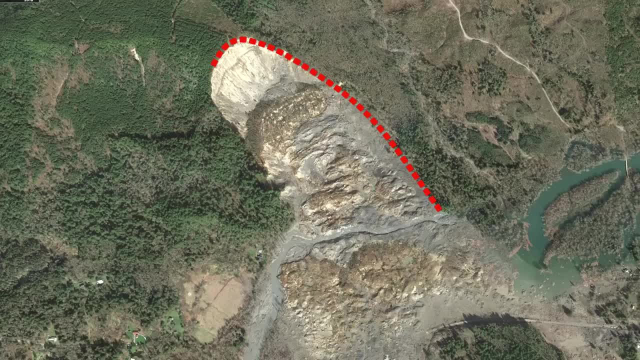 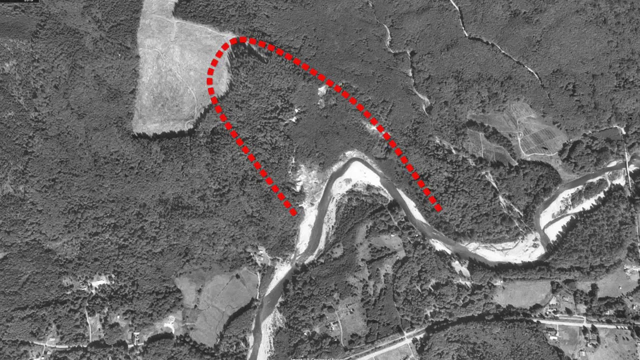 and I will show this line on images prior to the slide occurring. Let's start with this black and white image from 1989.. You do see a few bare spots that are suggestive of active sliding occurring In this image from the year 2005,. 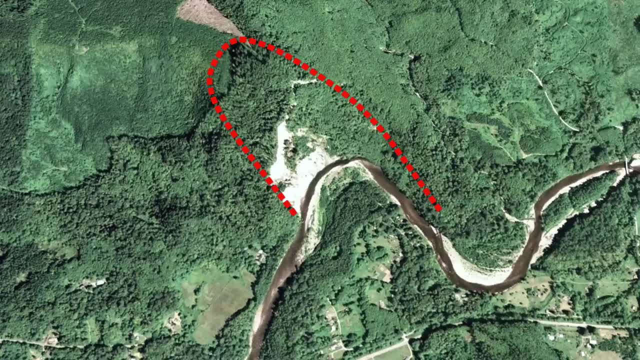 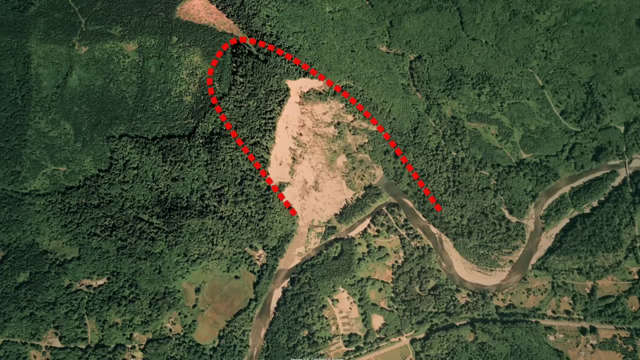 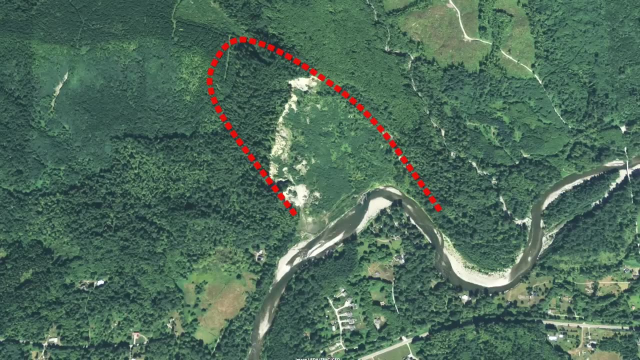 you can clearly see a large bare area where mass movement is occurring, which is destroying vegetation. In the year 2009,. the area of active movement increased dramatically In the years 2011 through 2013,. things seem to improve, with vegetation reclaiming much of the active slide area. 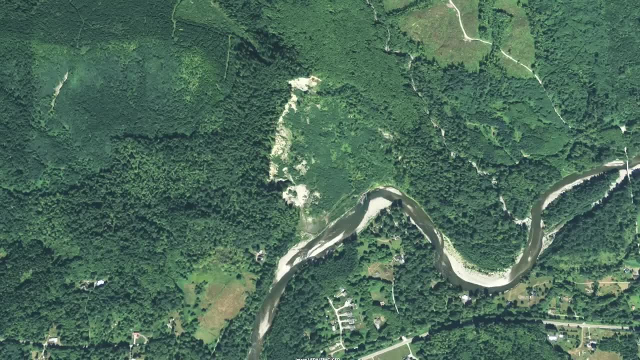 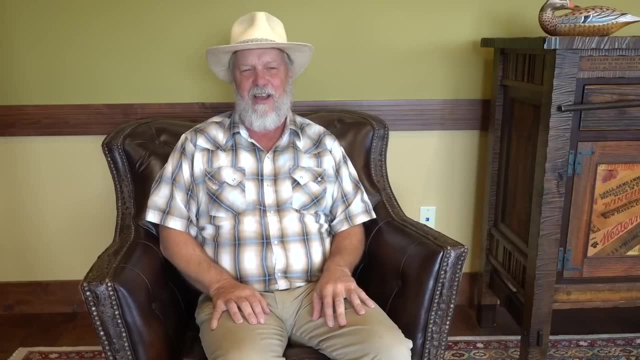 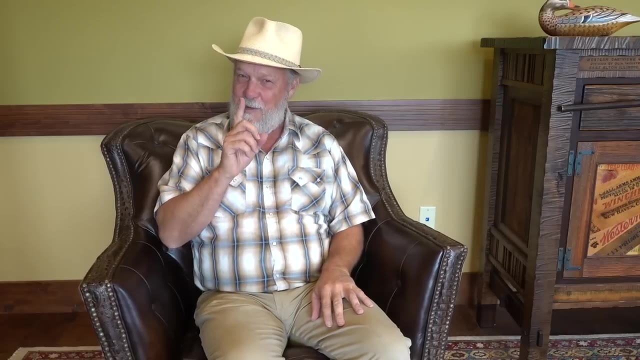 It's hard to believe that such a huge landslide was soon to occur. I hope you're beginning to feel some confidence in your ability to recognize areas that have potential landslide risks, And I'm going to give you one more chance to practice your skills in this. 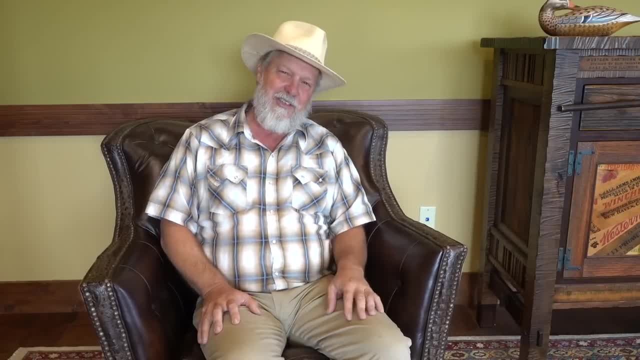 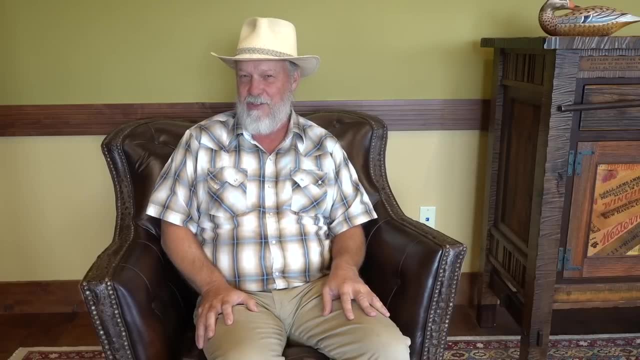 Remember those two hypothetical home locations that we talked about earlier? Well, I'm going to have you look at the drone video that I acquired over those locations and see what you think. But first I want to back out and think about the bigger geology picture. 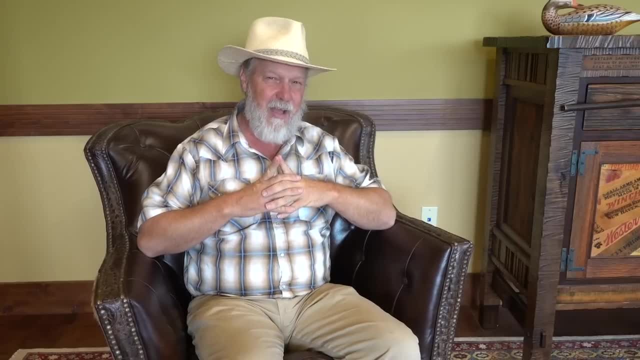 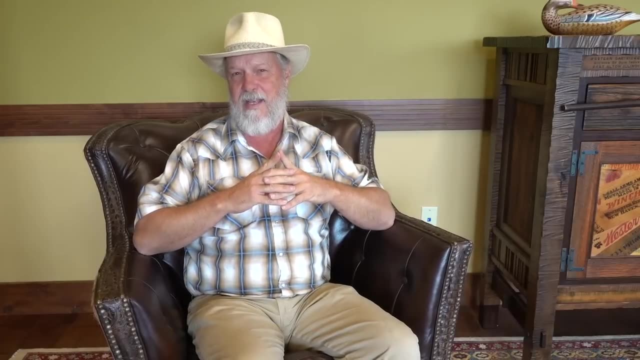 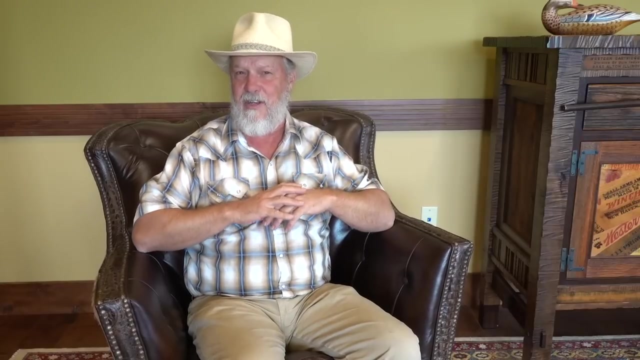 You know, these processes that we've learned about can occur on a grand scale and tear down entire mountains and reform the landscape in dramatic ways. It reminds us just how dynamic our Earth is. Let's go to Colorado and see a great example of this. 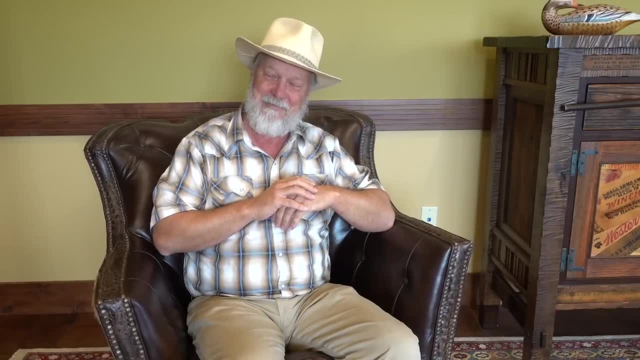 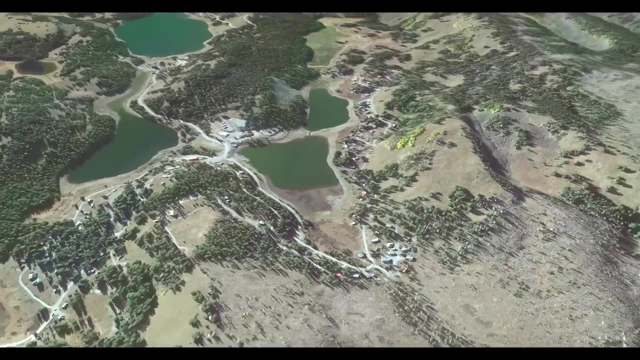 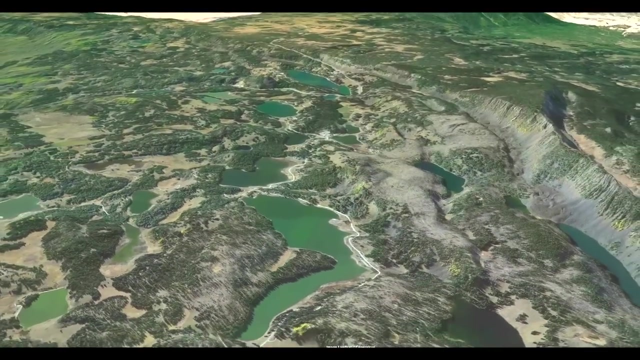 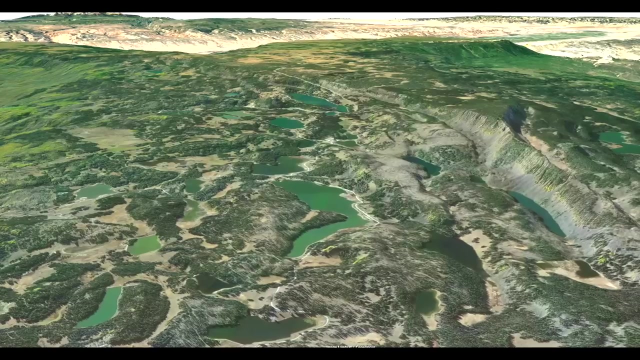 and then we'll review our two home locations. This is the Grand Mesa area of western Colorado. There are sure a lot of natural lakes here aren't there. I think these lakes are on the backsides of huge slumps and rotational blocks. 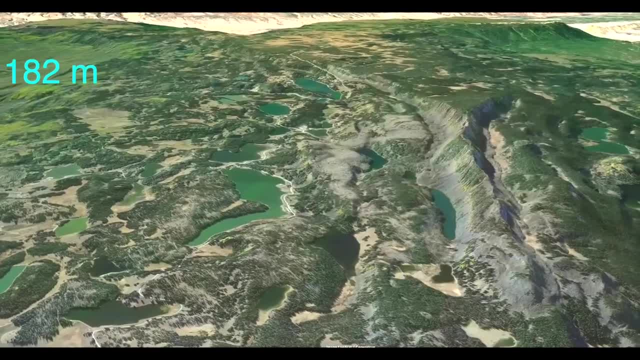 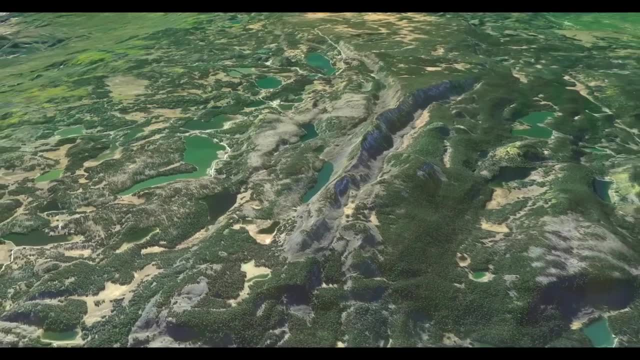 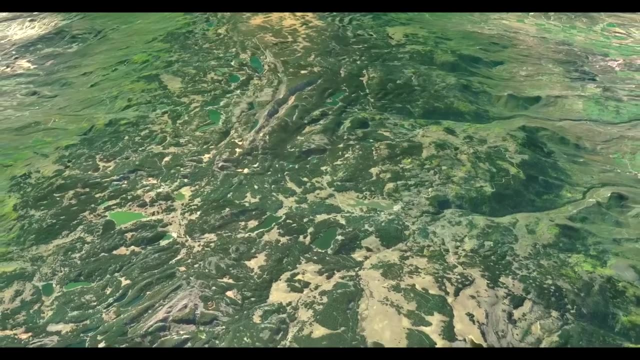 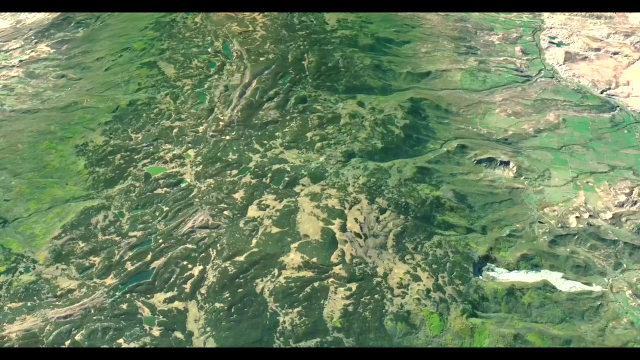 This massive scarp is about 600 feet tall. Zooming out, we can see that this mass wasting occurs over a huge area. The width of the area affected is about 10 miles and the length is some 25 miles long and goes beyond the view here. 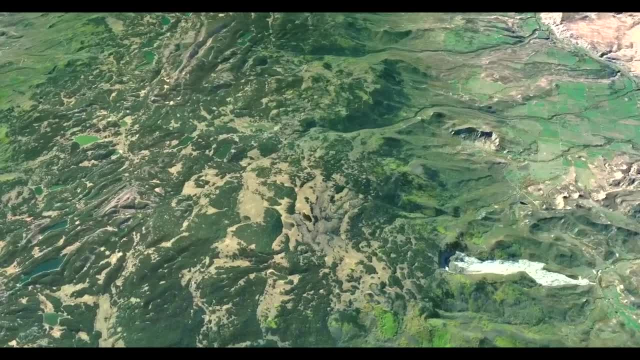 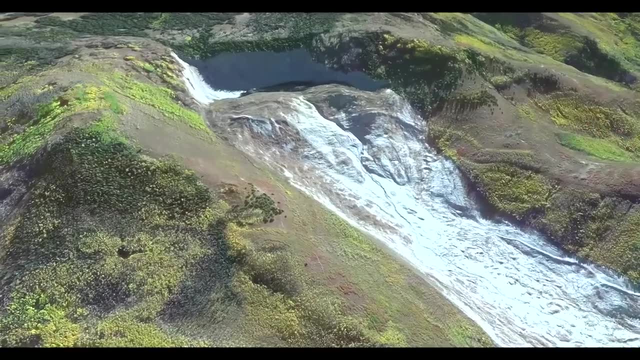 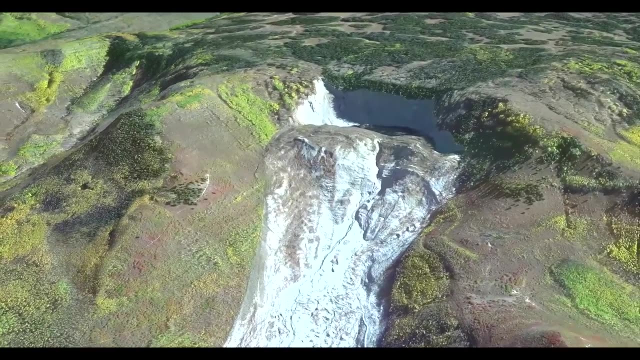 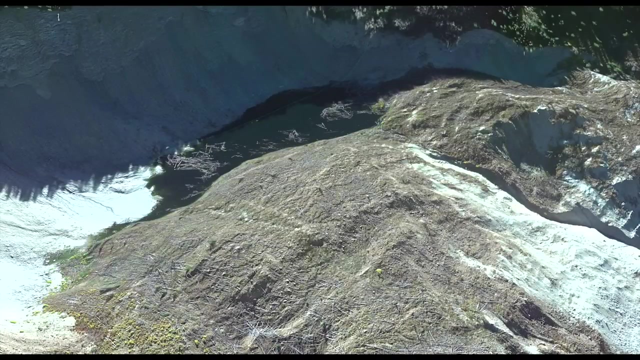 This massive slump with a debris flow below it is about 2.5 miles long and killed three people in 2014.. Here we see huge numbers of dead trees on the slump and the lake that formed behind it. It's time to look at the drone video.